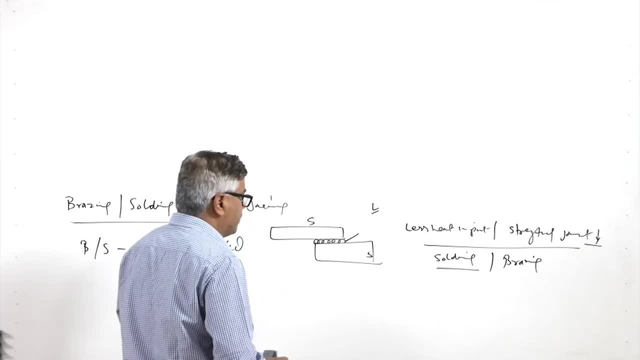 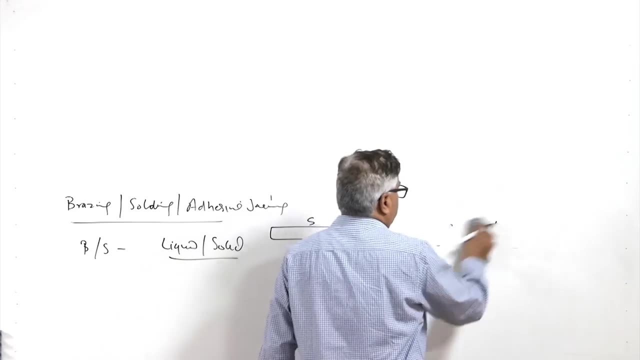 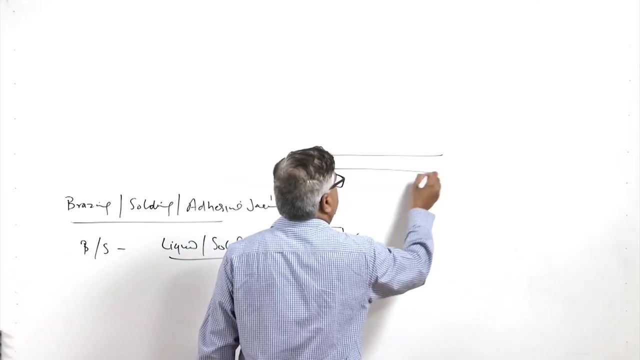 So the stress and strength requirements are not much high. So under those conditions the brazing and shouldering is found to be very effective. There is another process which is called adhesive joining, where, in the chemical reactions between the adhesives and the functional surfaces, this faying surfaces of the joints to be made. 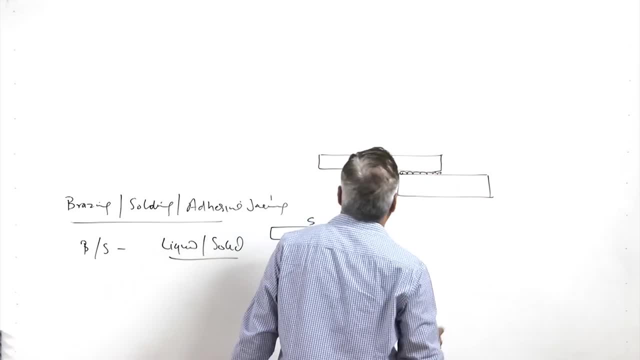 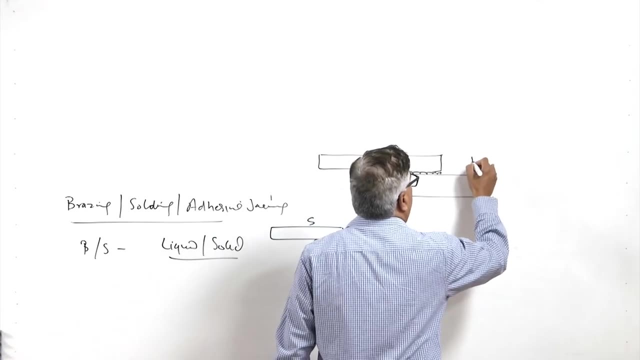 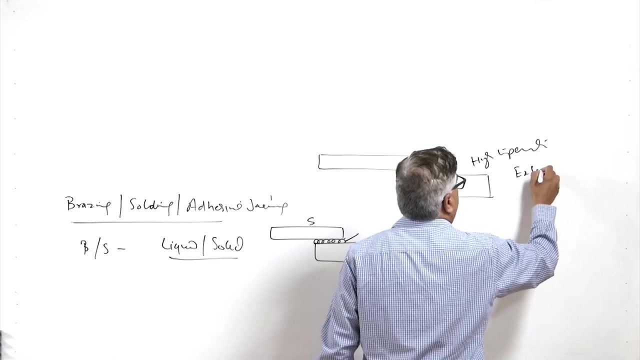 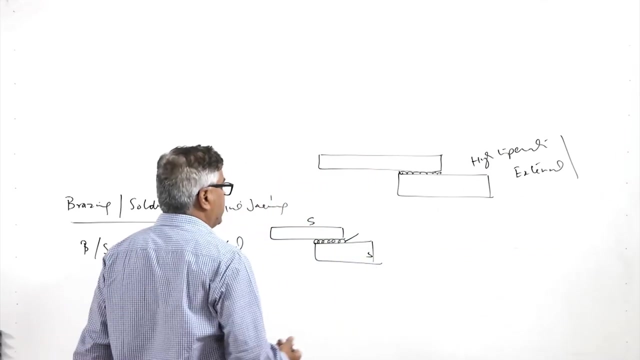 in, So adhesive is placed in that case. Normally, structural adhesives are used for high strength joints, but these cannot be used for the high temperature conditions and even for the external environmental conditions because these, under these two conditions, the adhesive tend to degrade and the joint is not. 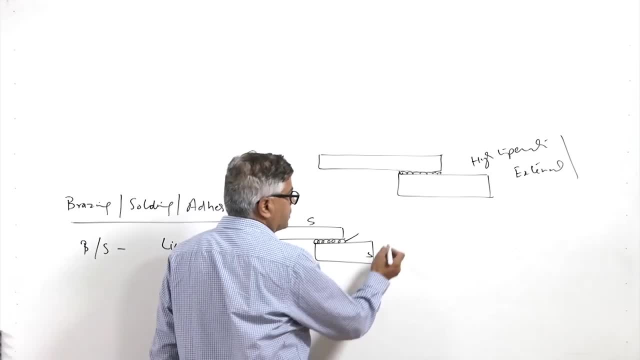 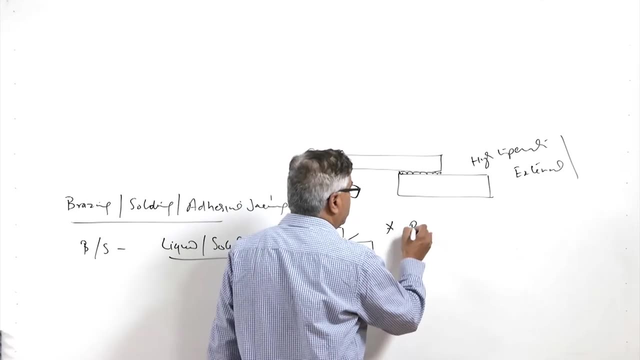 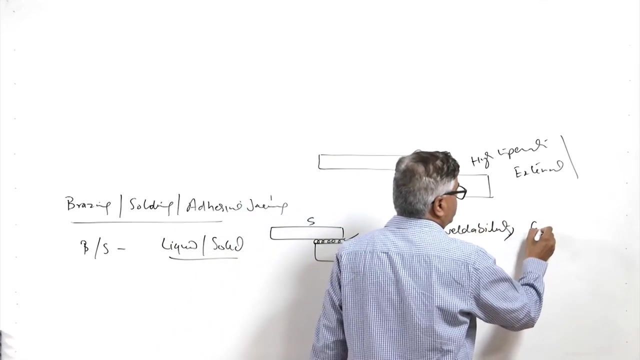 is weakened very badly. So the conditions under which the brazing joints and shouldering joints are preferred include like: where the fusion welding is not possible due to the poor weldability. Due to the poor weldability, the fusion welding is not a workable option. 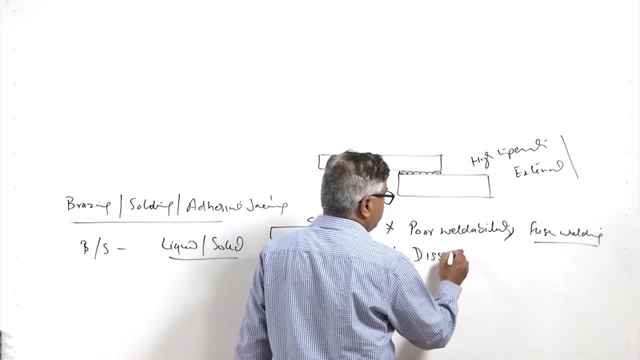 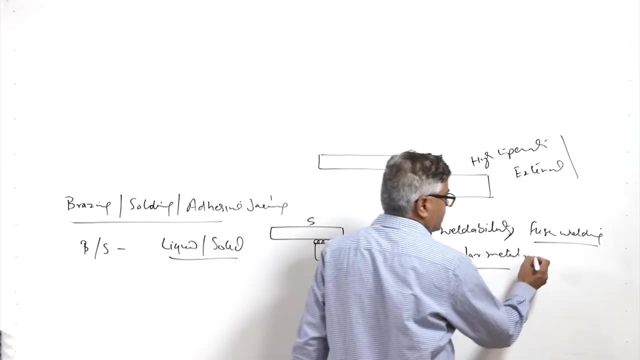 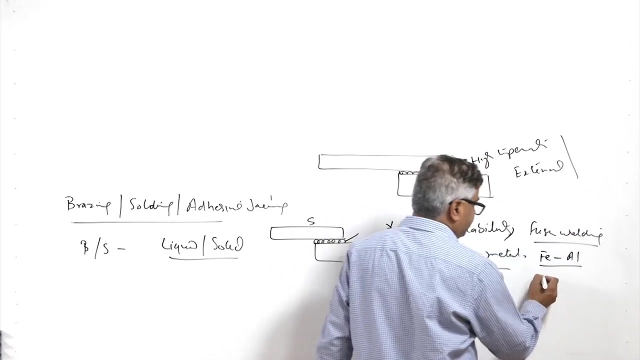 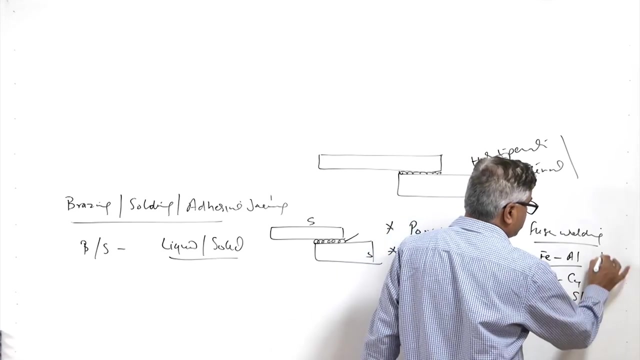 The second is completely different. metals, like dissimilar metal systems need to be welded where the compatibility between the two does not exist, For example, like there may be iron base alloys and aluminium, or iron and copper, titanium and steel. So these are the systems which are, if they are not metallurgically compatible due to 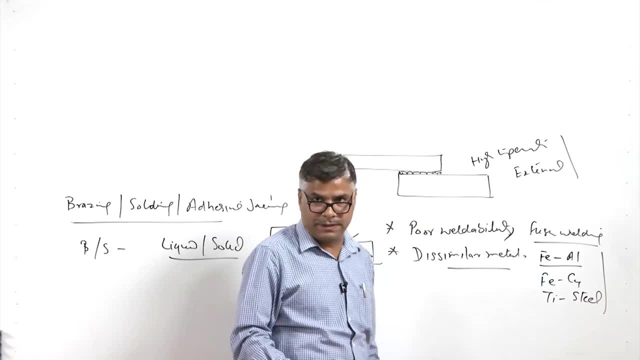 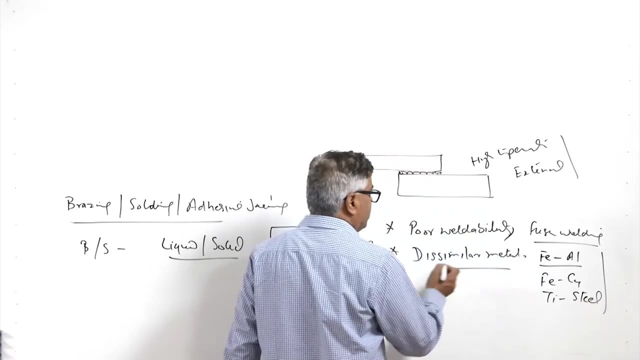 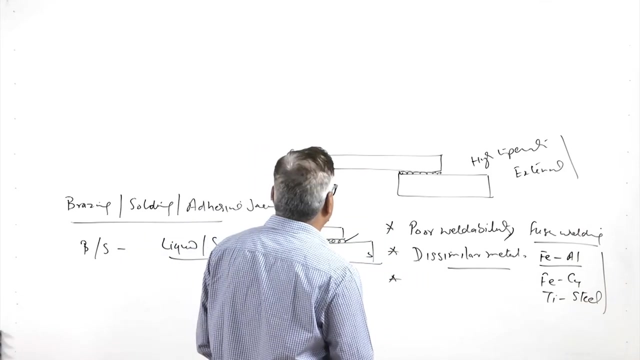 the variety of regions, like difference in melting point, expansion coefficient, yield strength, So they create lot of problem during the fusion welding. That is why Similarly dissimilar metal joining can be facilitated in number of cases through such kind of the joining processes where the base metal remains in the solid state, only the 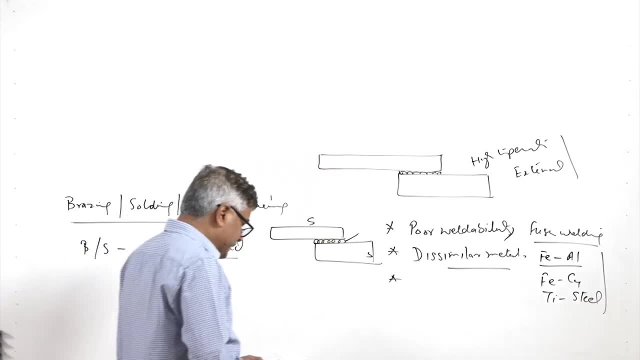 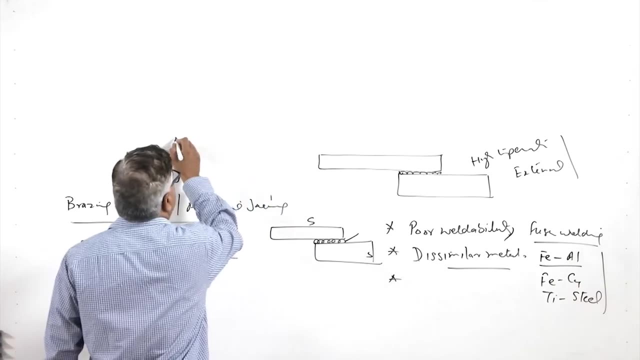 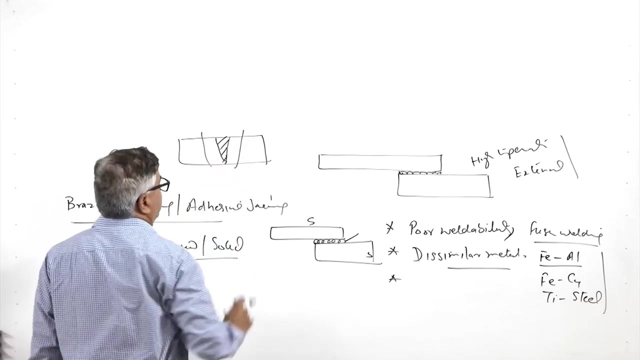 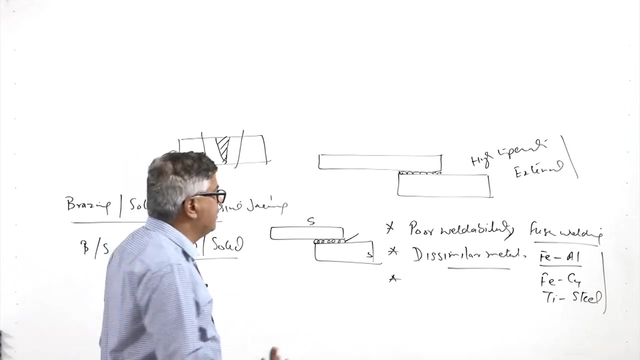 filler metal is brought to the melting point and then we have the conditions like the heat affected zone. you know we have seen in the fusion welding processes: application of heat results in the fusion zone but nearby a lot of heat affected zone is formed which has a different properties in terms of the metallurgical characteristics and the mechanical behavior. 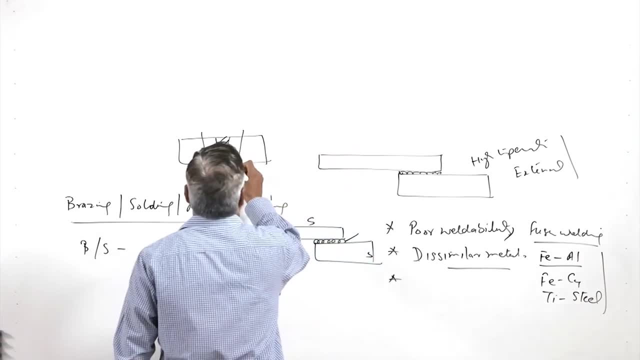 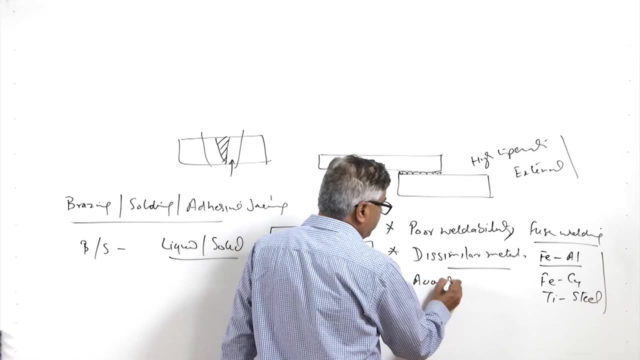 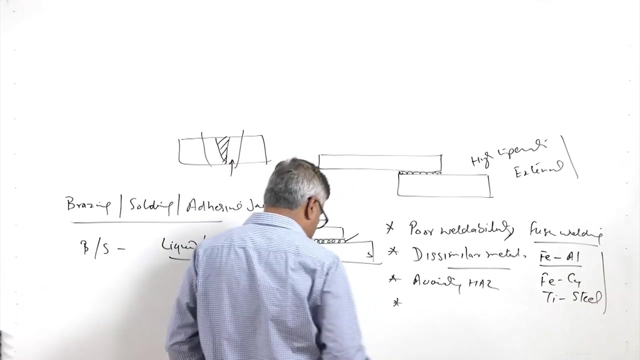 even the corrosion properties are adversely affected. So if the heat affected zone is unfavorable, which is produced in the fusion welding, So avoiding the heat affected zone, avoiding HAZ helps when the brazing and shouldering processes are used and like even the low strength joint is ok. 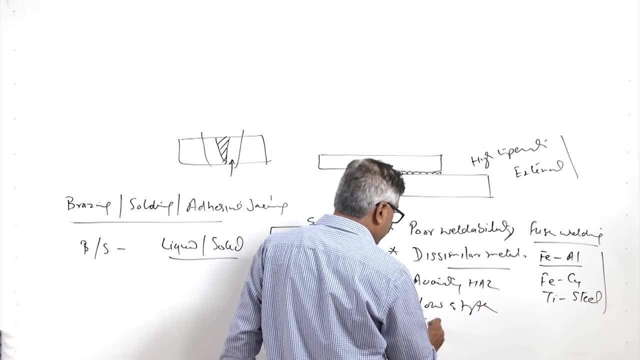 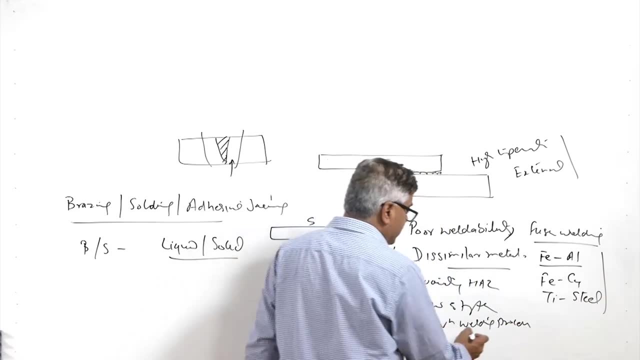 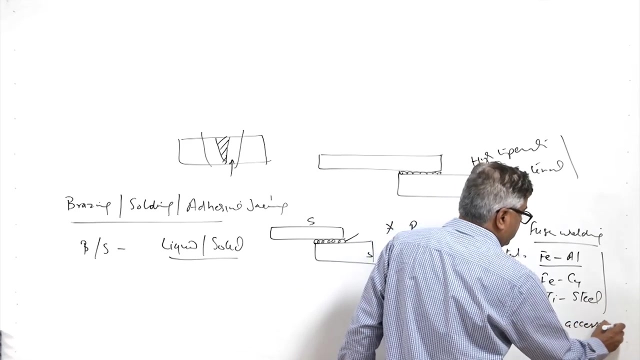 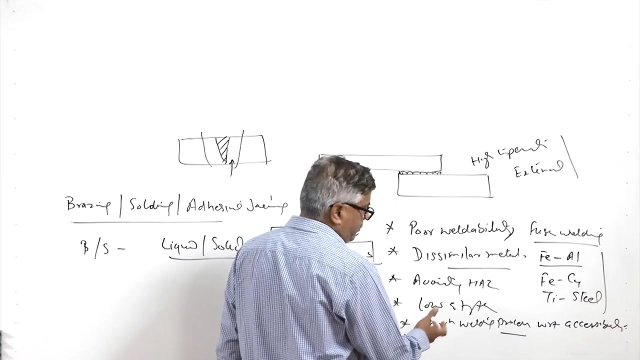 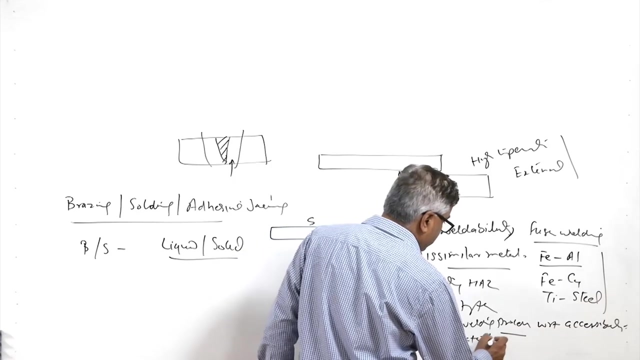 So this is the main problem. 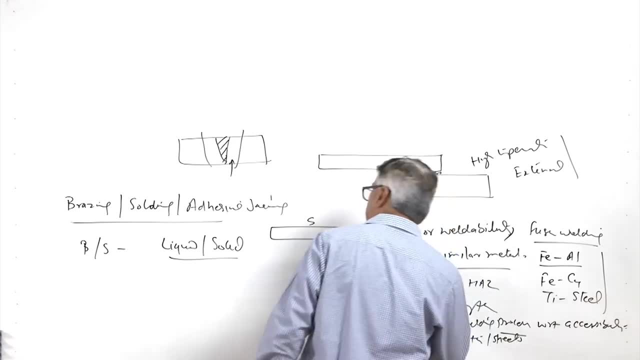 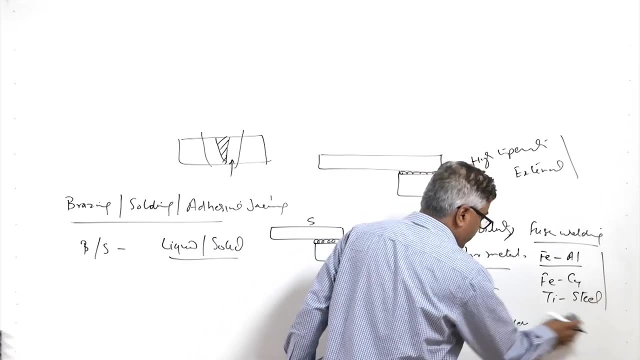 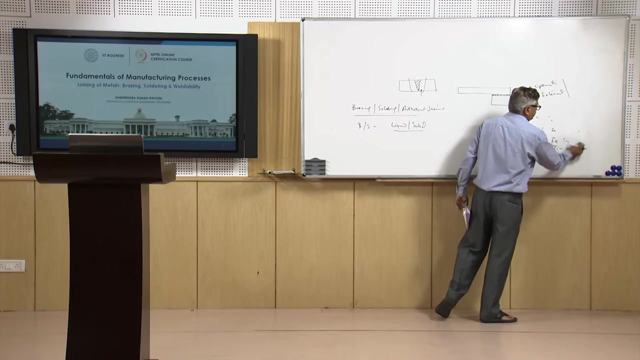 thin sheets need to be welded. there, the brazing and shouldering can be effectively applied for developing the joint, while the fusion welding may not be feasible and workable effectively. So for to deal with these conditions, the brazing and shoulder joints are used. 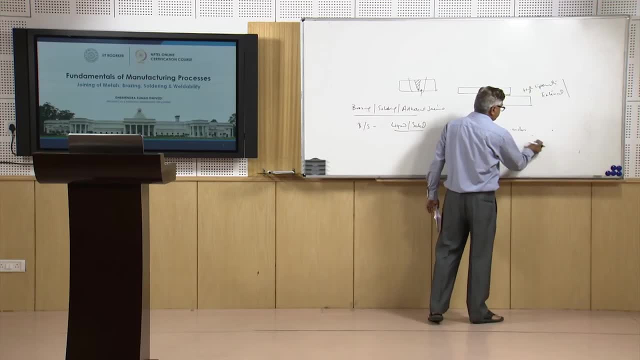 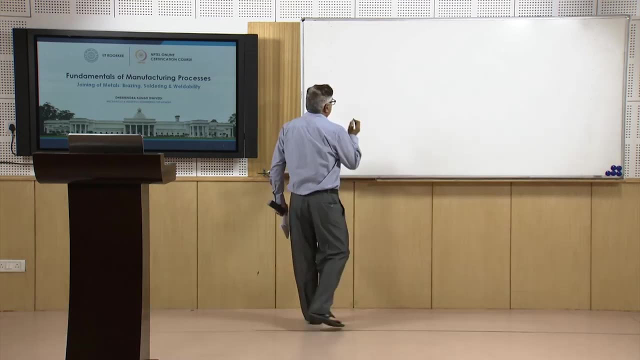 Now we will see the basic principle which is used in these processes in the development of the joints. So we will take up first the brazing joints for this purpose, like say, the plates to be welded are mostly there can be the different kind of arrangements wherein, like lap joint, 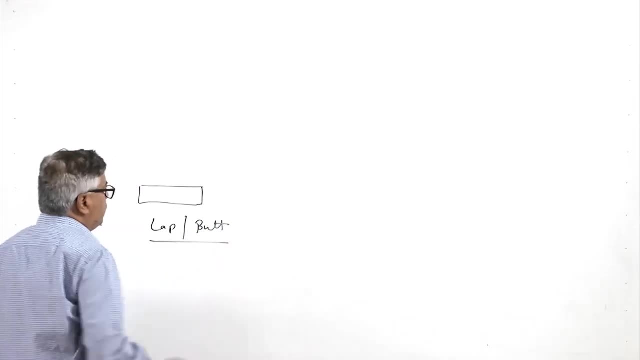 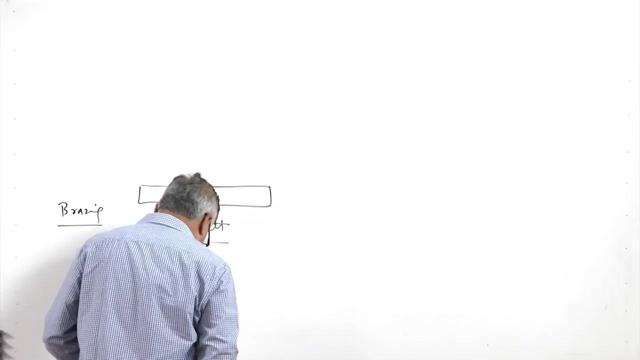 or the butt joint. both can be made, but it is more common to use the lap joint configurations for the brazing purpose And whatever. So So like say, this is the butt joint configuration and the different joint designs have been proposed for the butt joint configuration. 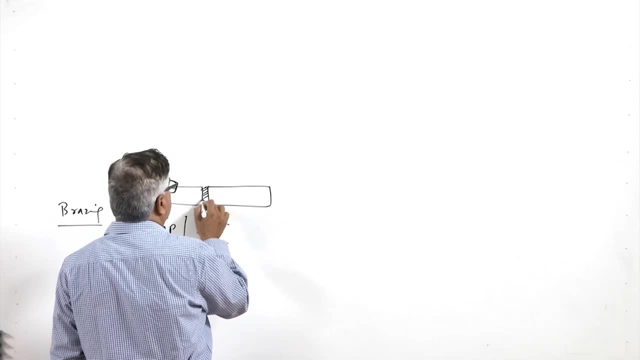 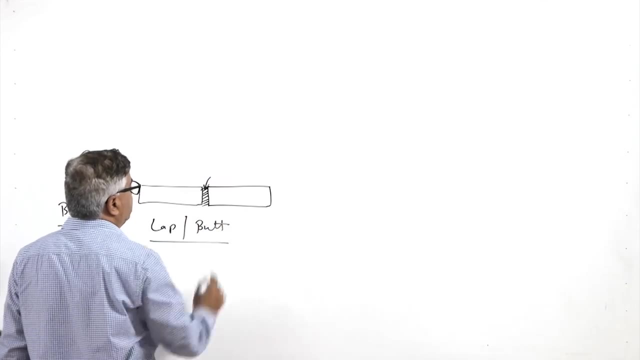 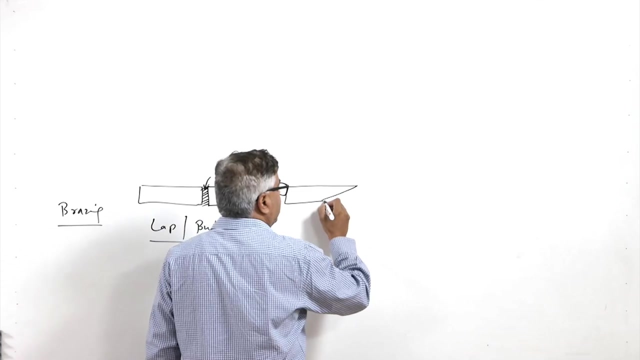 Here. this is the square one, but square one will be ok if, very if, the strength is not a middle criteria because the weld area is very limited. So in order to increase the strength of the joint- in this case some kind of the joint- 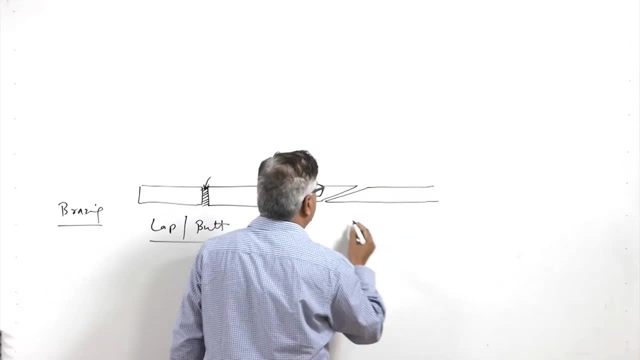 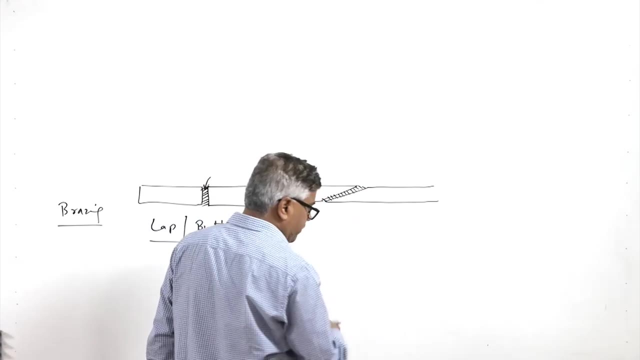 is prepared in such a way that the joint is not too tight, So the joint is not too tight, So the joint area is more so. such a larger joint area will be increasing the strength of the joint by making the faying surfaces at certain angle, another arrangement which. 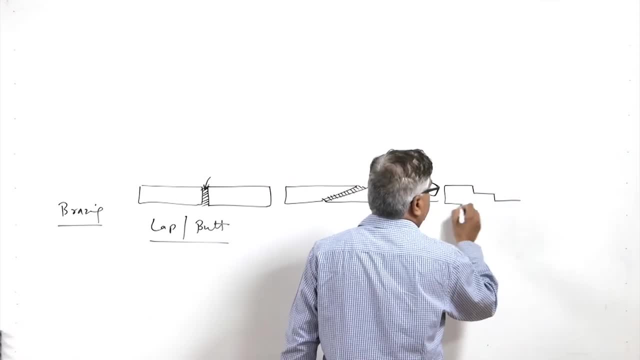 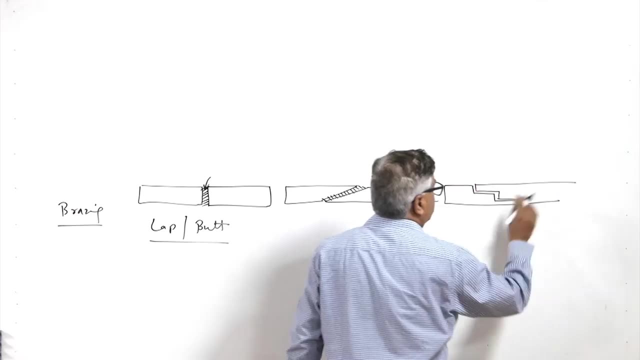 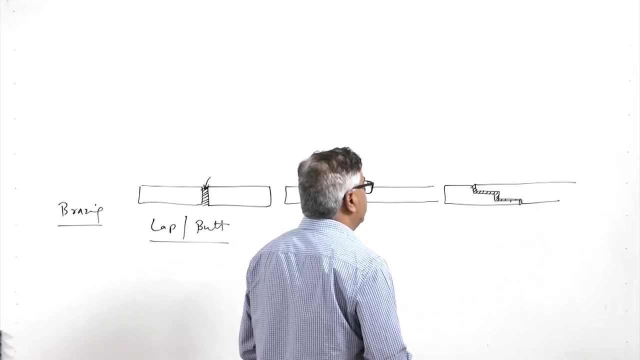 is. which can be made is like this: for developing the butt joint, like this- So this is also butt joint- and the faying surfaces, and in between the faying surfaces, the brazing, So the brazing joint, the brazing alloy is applied. then there is one another kind of 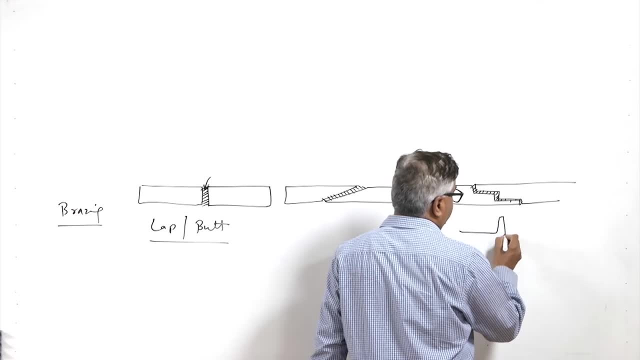 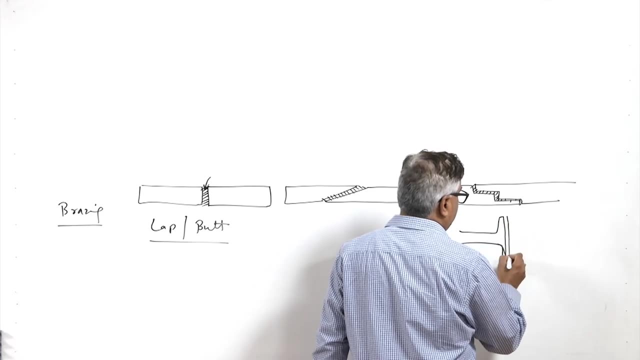 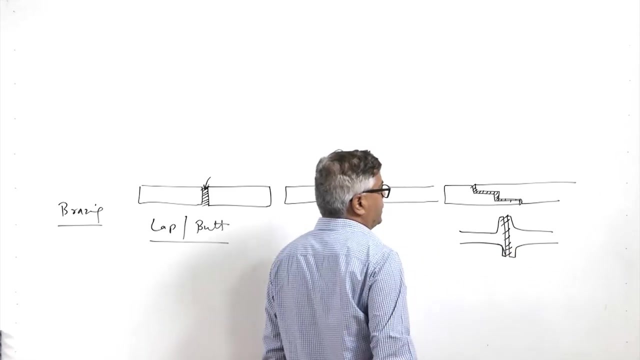 arrangement where, near the faying surfaces, the cross section is increased. cross section is increased like this, So that larger joint area can be achieved for having the desired strength. and here this is the location where brazing system will be applied, so increasing the strength in. 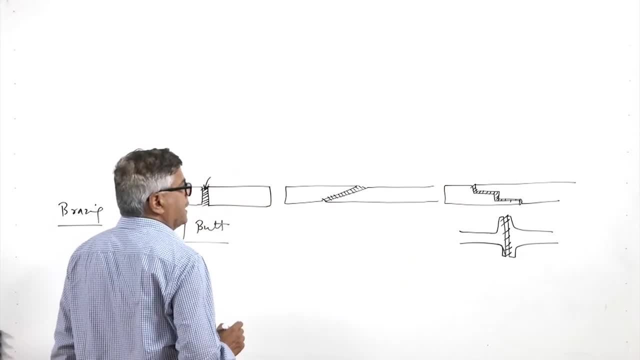 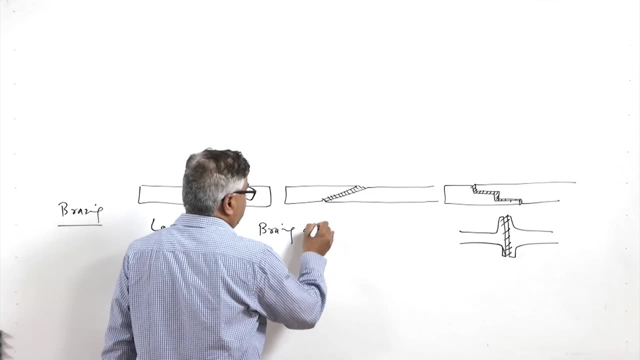 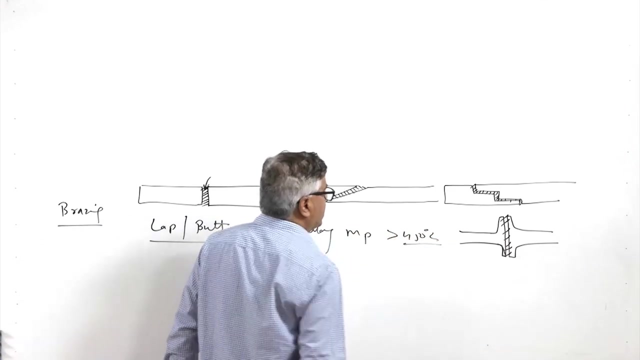 all these designs. So these designs is based on increasing the joint area for the brazing purpose. So for brazing. basically, the brazing alloys are used for brazing purpose. they normally have the melting point greater than 450 degree centigrade. but the issue with this is that 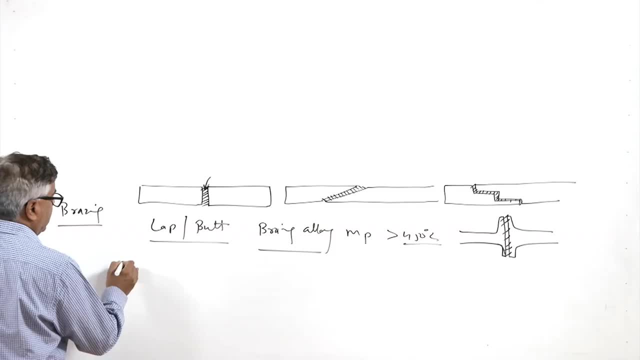 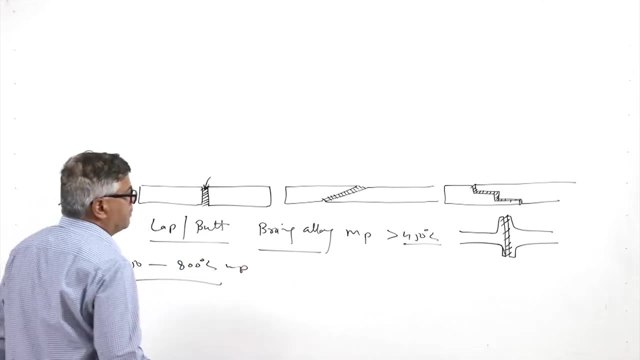 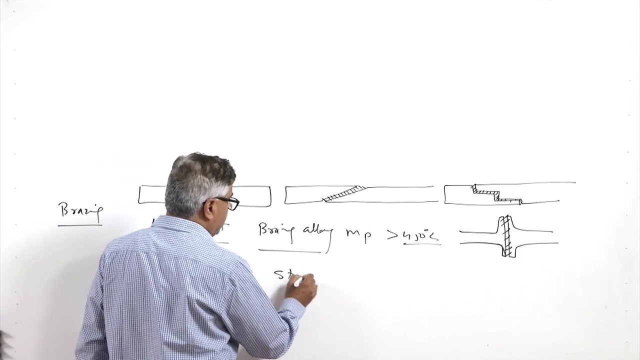 the brazing joint. generally they have, like the temperature, in the range of 450 to like, say, 800 to 900 degree centigrade In terms of the melting point. so if we compare, like if these are being used for joining of the steels, then strength of the strength of the brazing joint is lower. they are ableted. 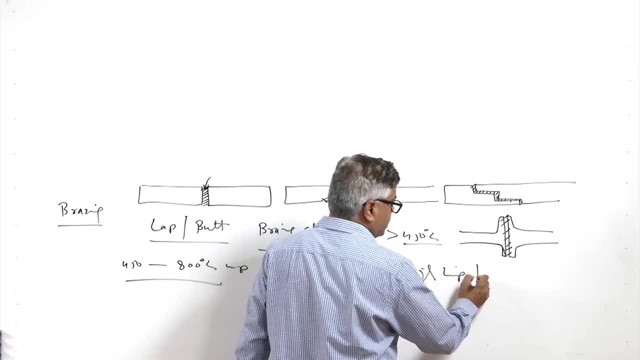 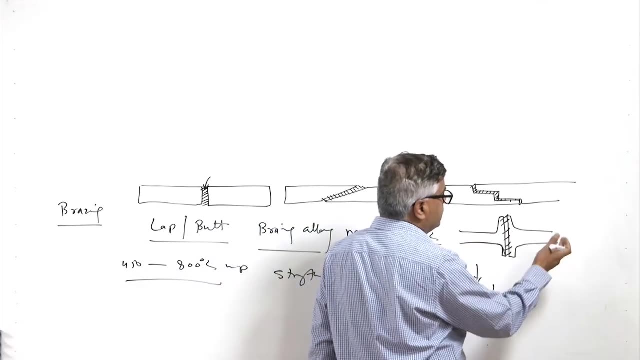 for the high temperature with standing is lower. they cannot with stand at high temperature as well as they sometimes, because the brazing material is different from the parent material. So galvanic corrosion is proposed. So the brazing material is different from the parent material. 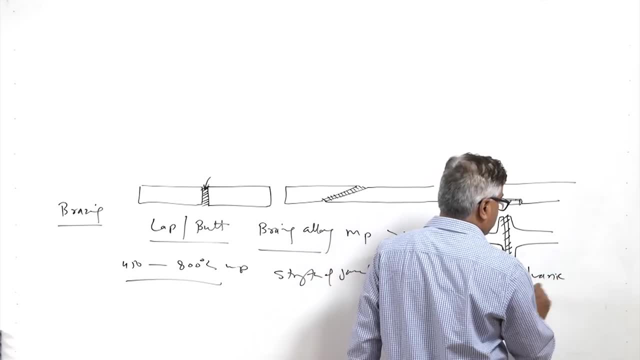 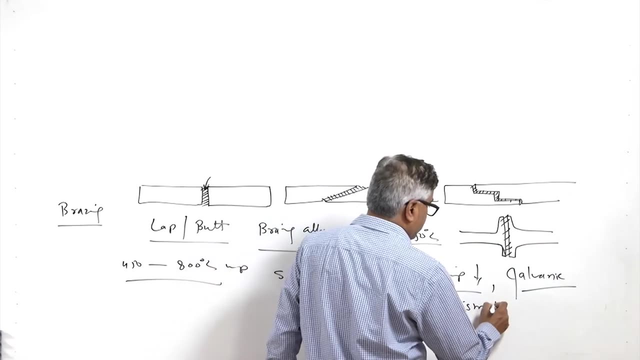 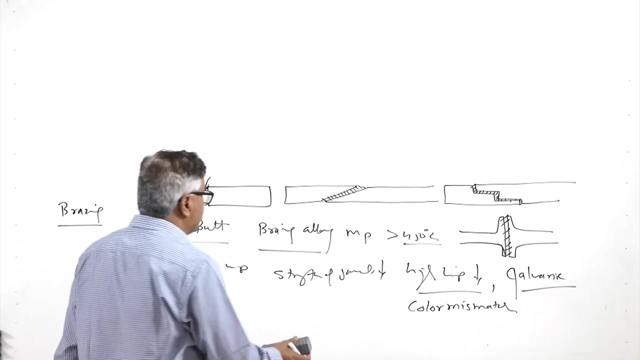 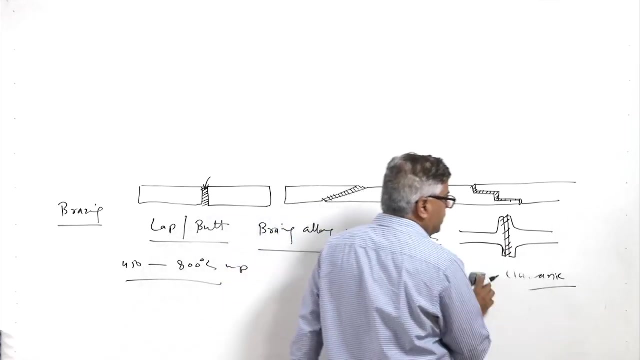 So galvanic corrosion is proposed. Galvanic corrosion is promoted by this and even colour mismatch is also observed when the brazing is performed. So these are the some negative aspects, apart from the benefits which are produced. like the joint is made with the reasonable strength without melting of the base, metal limited 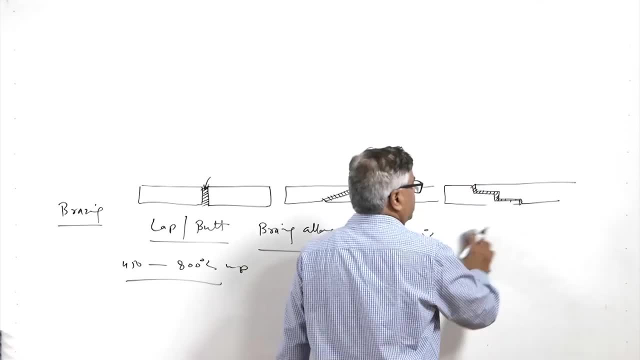 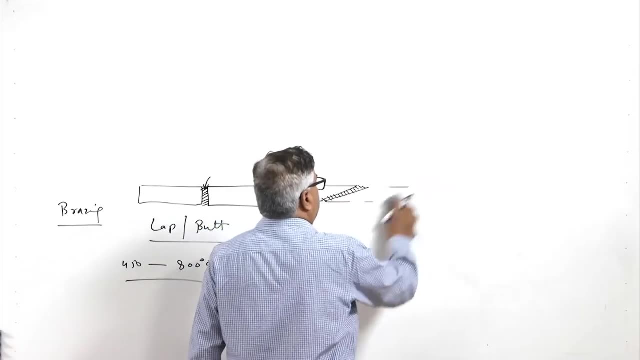 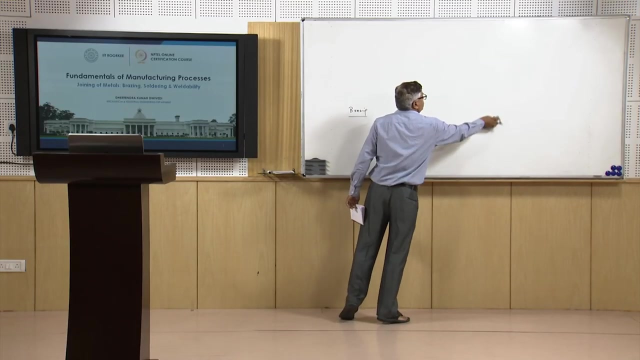 heat input. limited size of the heat affected zone. So there are so many benefits. So there are so many beneficial aspects still related with the brazing. For brazing a special kind of approach is used where in the surfaces to be joined are. 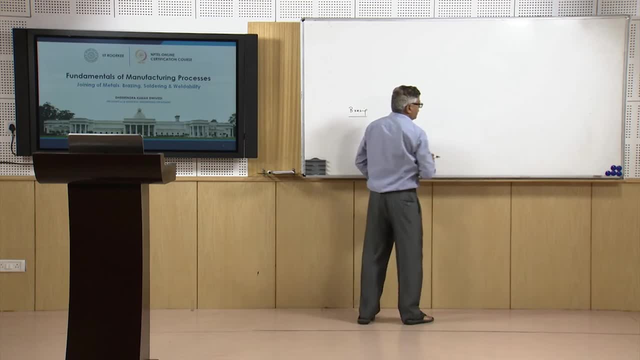 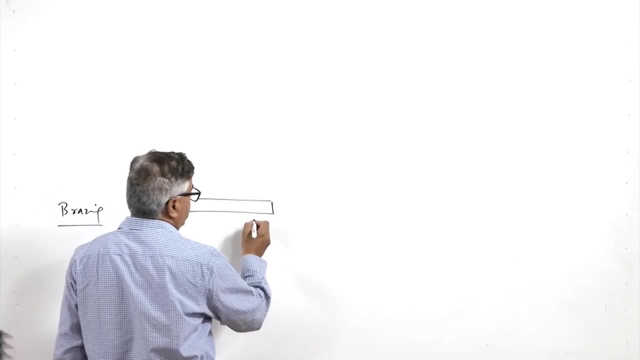 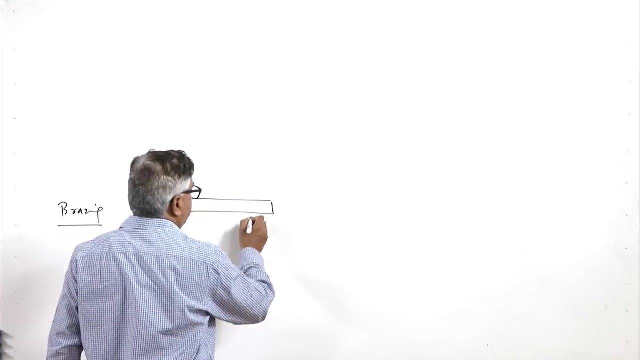 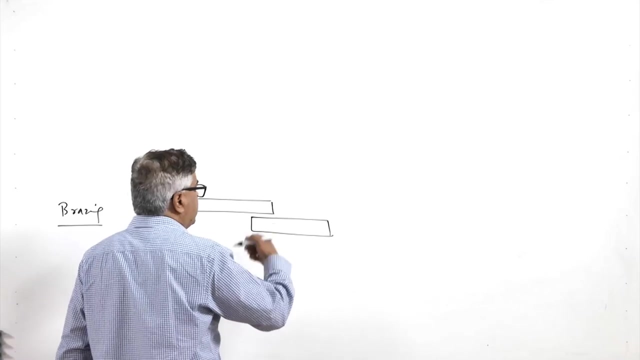 cleaned properly and they are smoothened properly so that the flow of the metal can be smooth, like say, in this configuration. this is the lap joint configuration, and various lap joint configurations are used here. One typical one is this one where in the surfaces to be joined are placed in overlapping position. 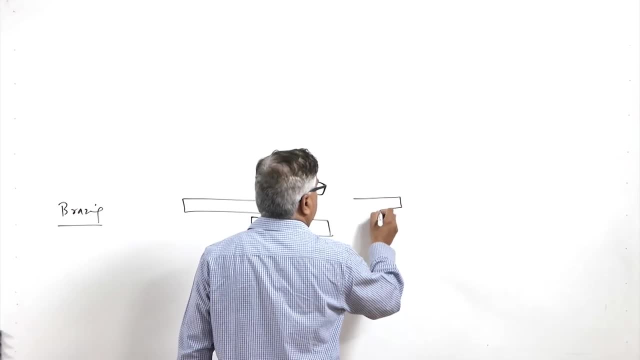 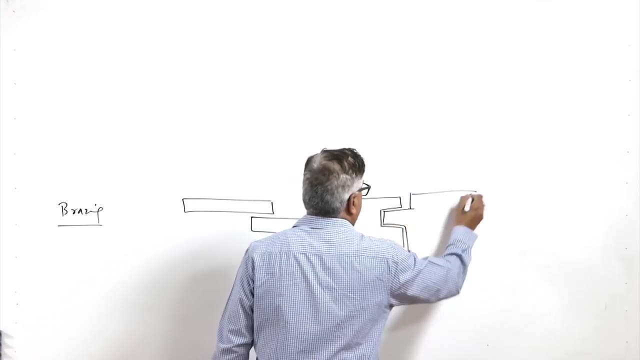 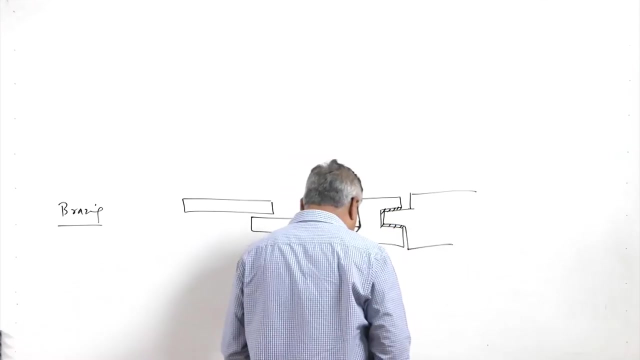 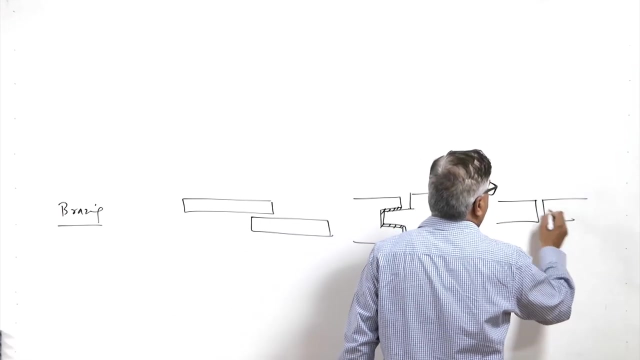 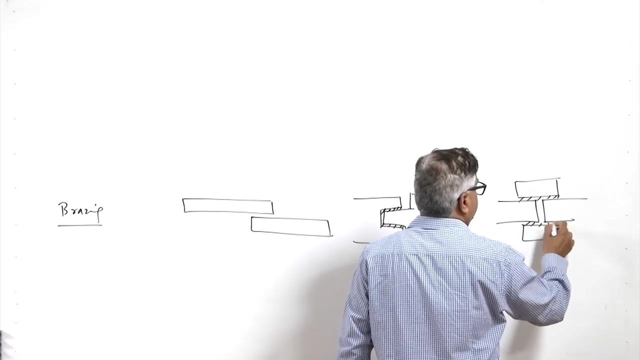 Another one is maybe like this: where in the components to be joined are kept in overlapping position, this manner, And here this is the overlap portion, And then there may be an arrangement where in the plates are kept both the sides in this way and the brazing joint is made like this, and then sleeve can also be used in this manner. 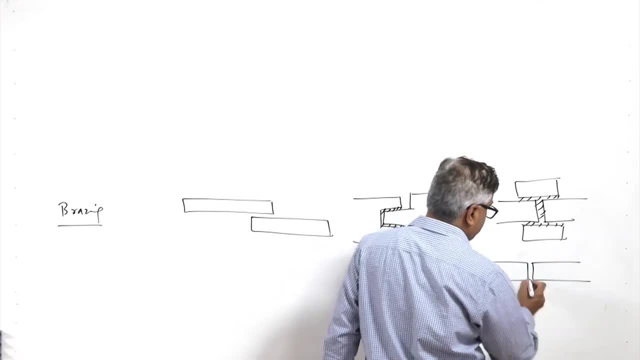 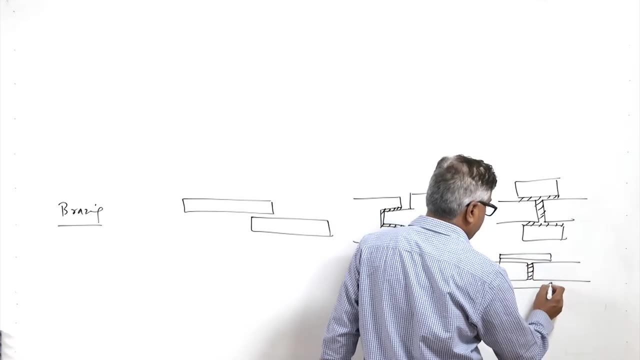 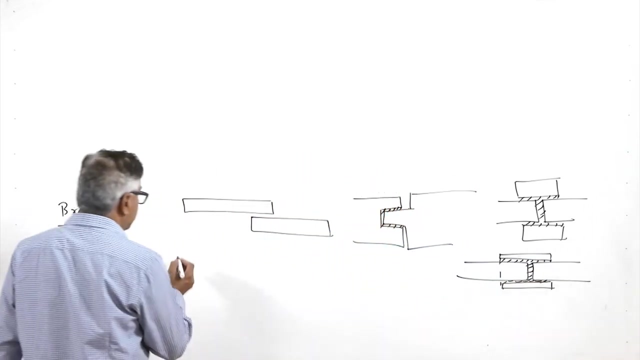 where the like say the rods to be joined in this manner. So brazing allowably placed here and then sleeve on both the sides is applied in this manner And here all this area is brazed. So for brazing purpose the important thing is surface cleaning. 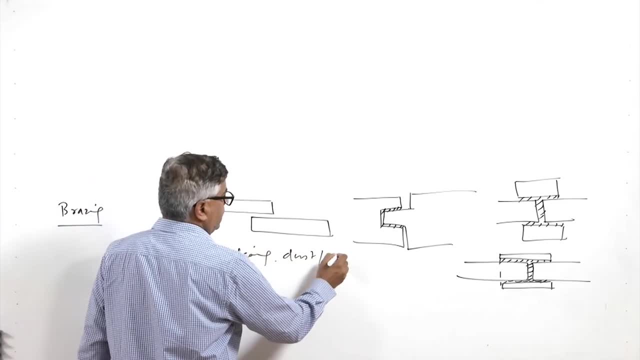 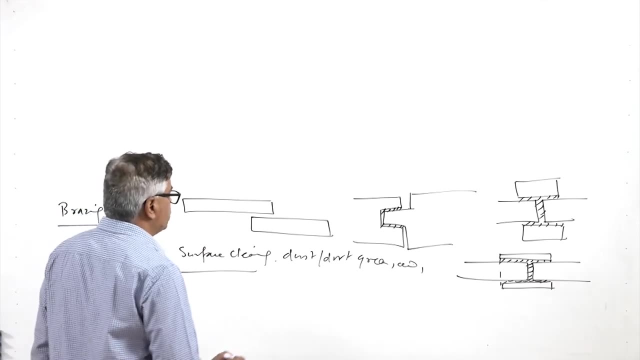 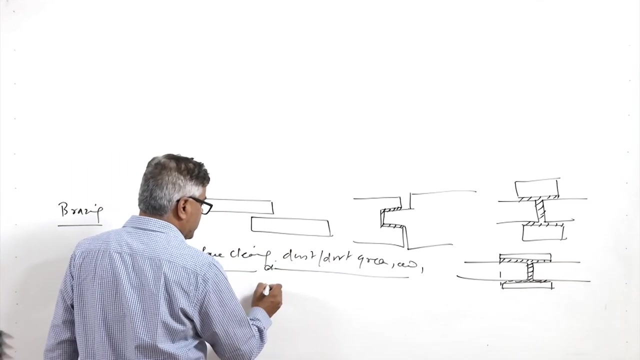 Surface must be clean from the dust, dirt, grease, oil, paint, etcetera, because these are the impurities which will be hindering the flow of the molten brazing alloy. and, apart from this This should the surface must be smooth enough because the molten metal has to flow through. 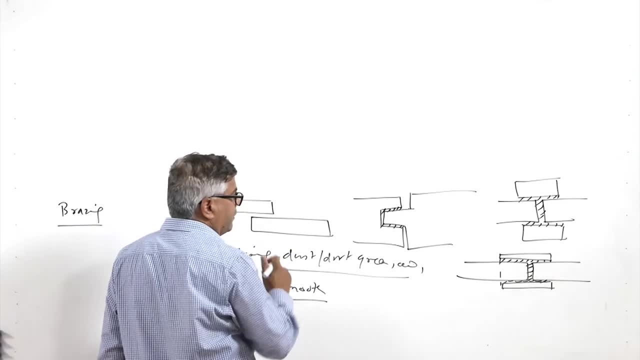 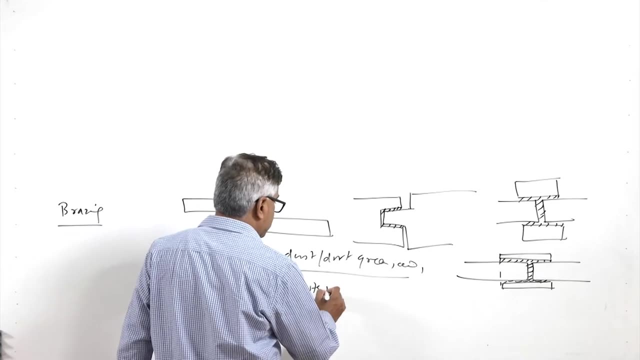 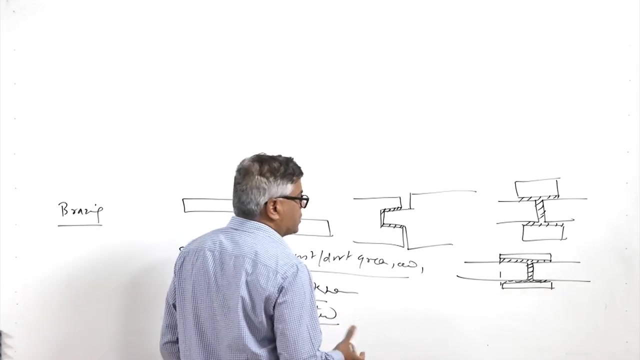 under the capillary effect between the faying surfaces in order to get uniformly distributed, And so the smoothness and the cleanliness is important. Thereafter it needs to be heated to the proper temperature so the they can reach to the melting point. 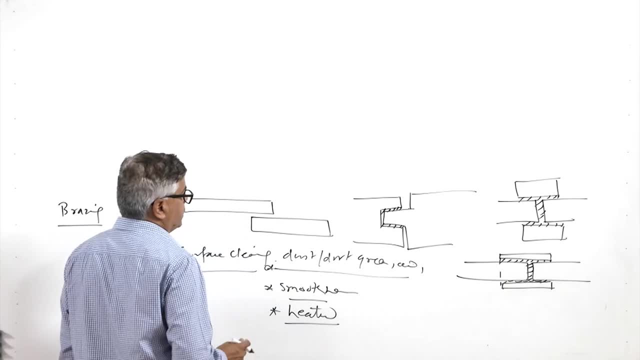 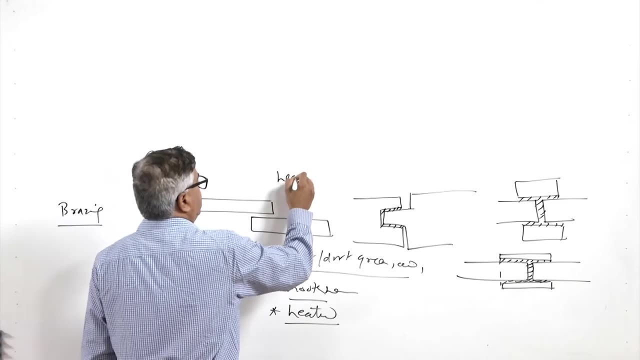 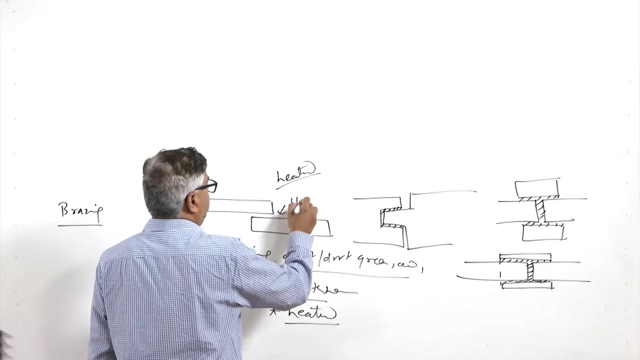 So what we do, basically say, this is the kind of arrangement which is to be brazed. So here, the plates to be weld brazed will be heated, the clean and smoothened surfaces will be heated, and then may be flux is applied, which will help in improving the removing. 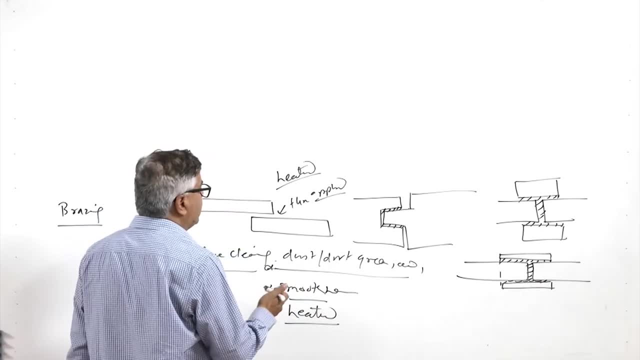 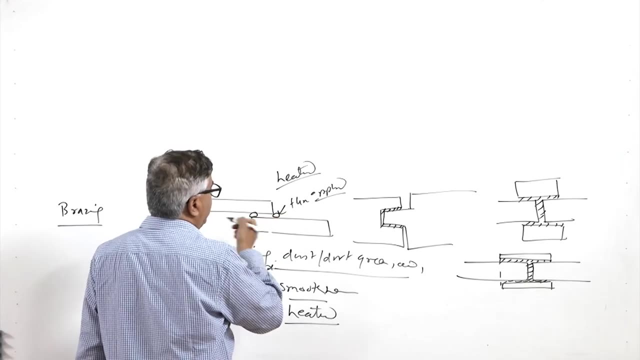 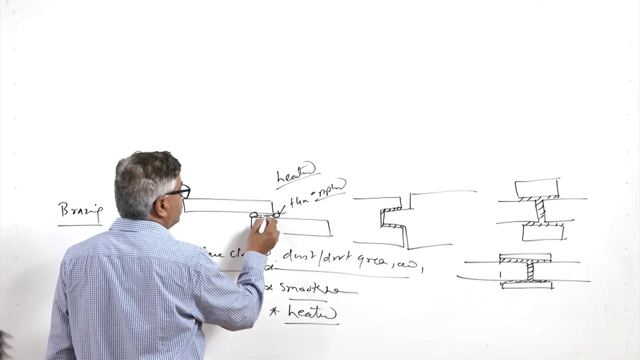 the oxides and facilitating the wetting of the brazing material. material is applied here like this: So it melts and due to the, and then it flow it by the capillary action, it is sucked inside and gets uniformly distributed. So for having 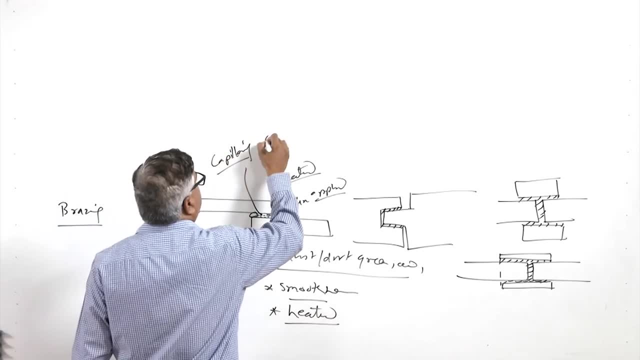 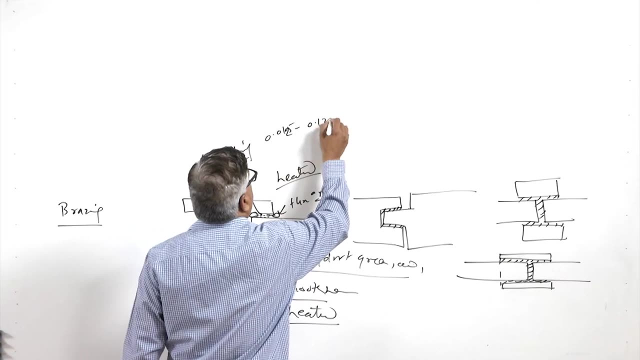 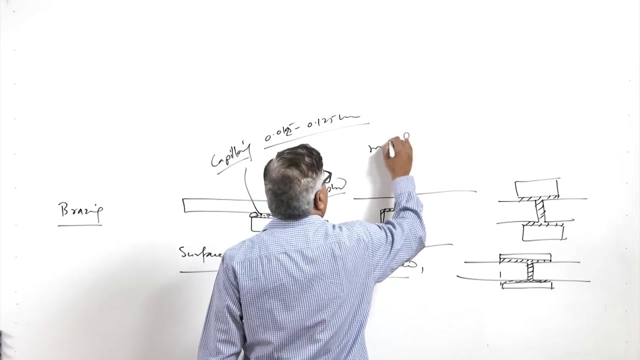 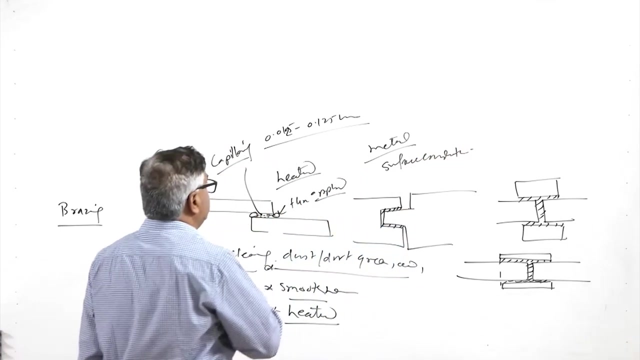 this capillary effect. what is important? that the gap between the two is very closely maintained. 0.0125 to 0.125 mm kind of the gap is maintained and this will be depend upon the metal of the brazing alloy, the kind of the surface conditions which exist at the surfaces and 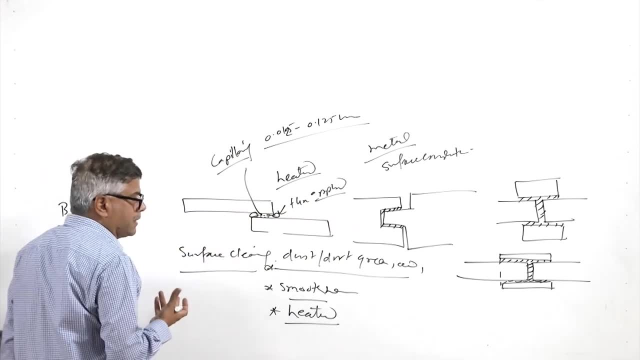 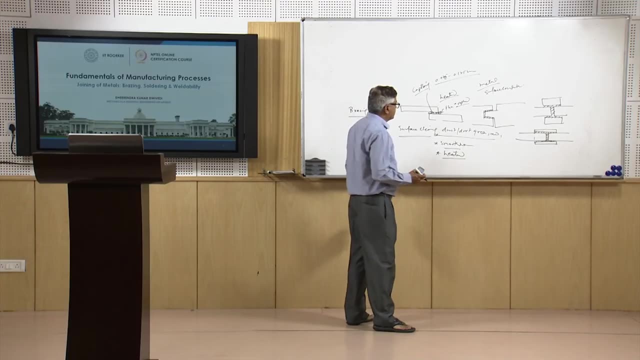 the cleanliness. So since the flow is here by the capillary action or distribution of the brazing, molten, brazing metal between the faying surfaces by the capillary action. So cleanliness is smoothness And a proper fluidity and wetting of the surface by the brazing material is important and flux. 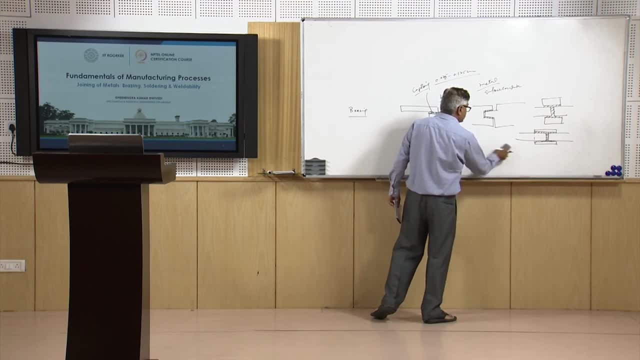 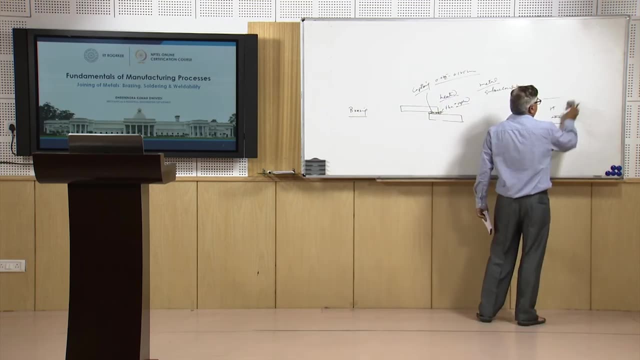 to some extent helps in removing the oxides and improving the fluidity of the brazing materials So that it can spread uniformly between the faying surfaces in order to form the joint and, after the solidification, the joint is produced. The common kind of material which is used for the brazing material is the material which 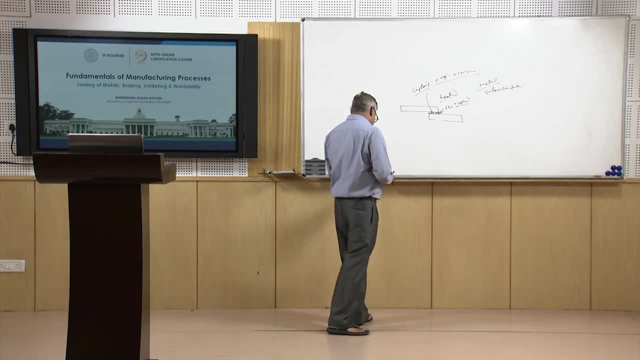 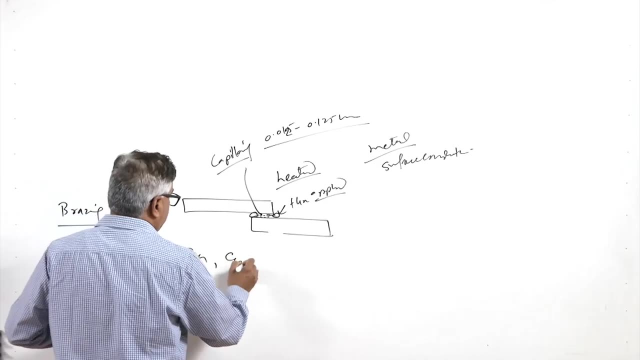 is used for the brazing material. So the material which is used for the brazing material is called theation. The brazing materials which are used- brazing alloys- are like copper, zinc, copper, tin, then copper, phosphorous and the nickel base. 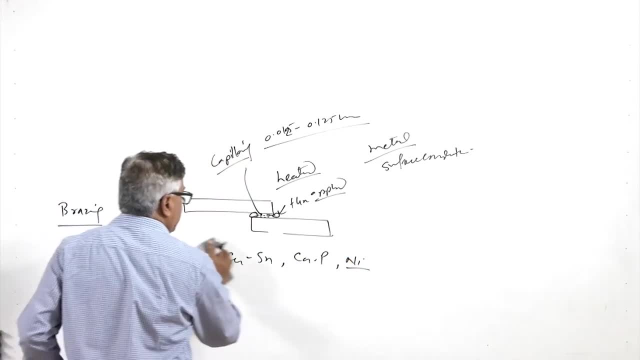 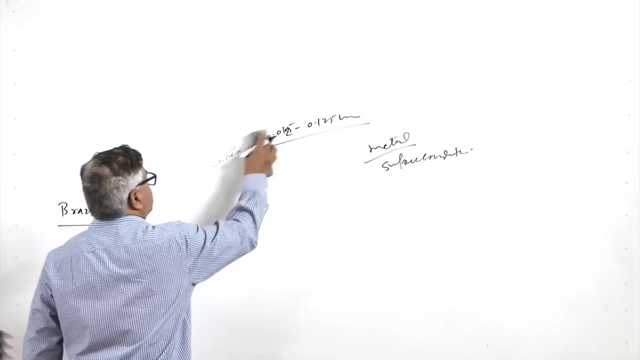 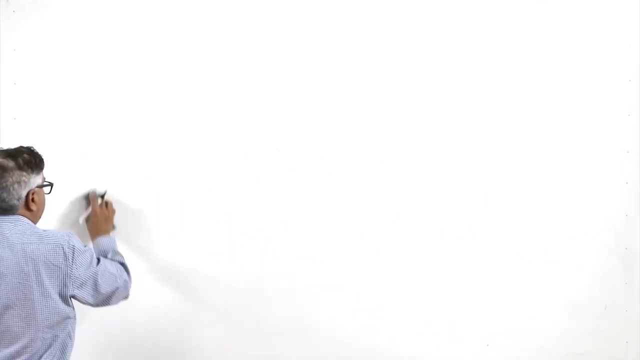 alloys are used as a brazing material, The compared to the shoulder joints. the brazing joints offer much better strength as compared to the shoulder joints because the shoulder use the filler metals having the melting point less than the 450 degree centigrade. 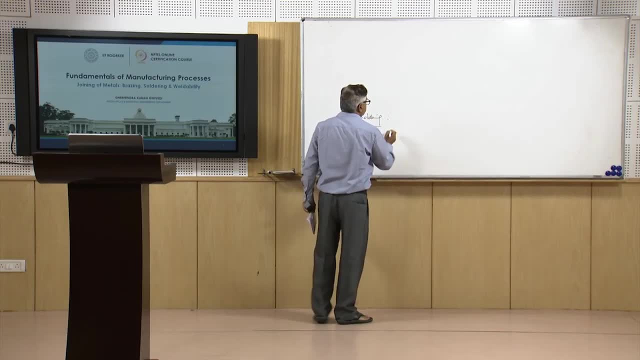 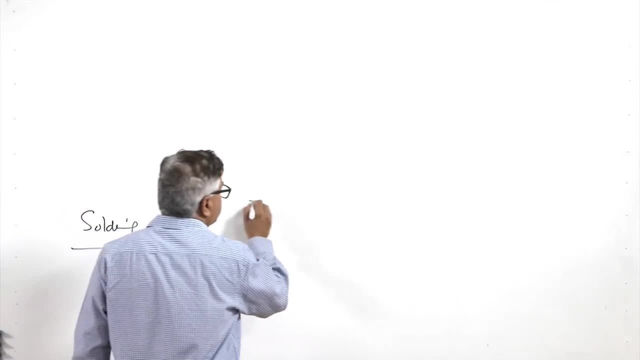 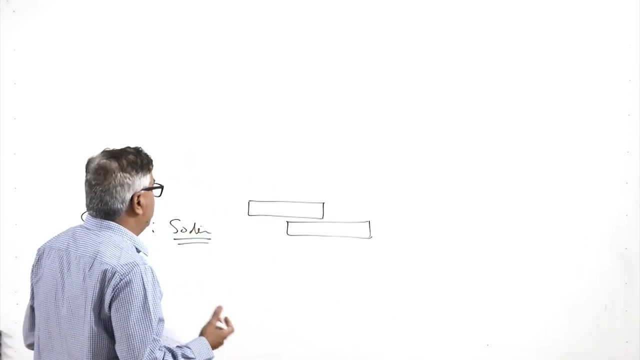 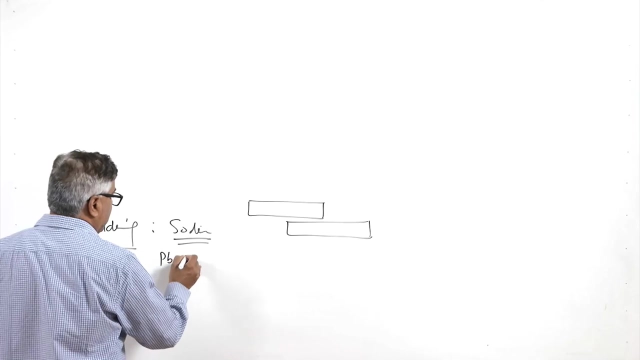 So next is the shouldering. So shouldering basically uses the shoulder for the joining purpose. The principle of this is same as that of the brazing, but it is of the much weaker, much lower strength and melts at much lower temperature. For the shouldering purpose, various kind of the shoulders are used, like lead, silver. 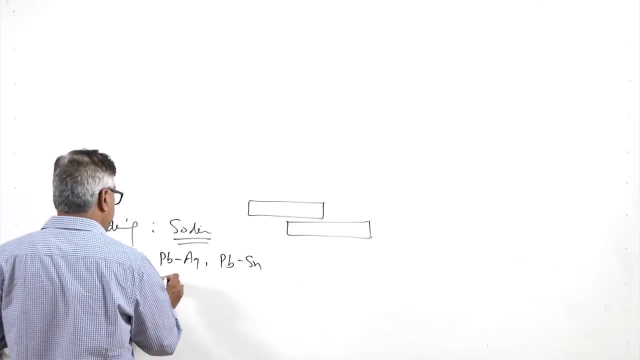 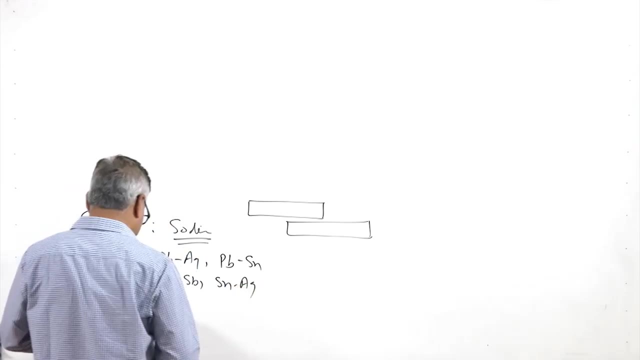 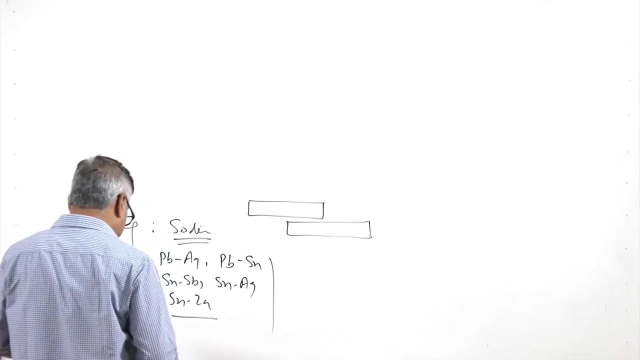 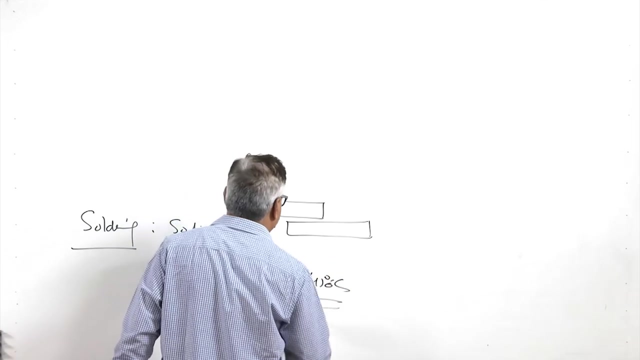 lead, tin, tin, antimony, tin, silver, tin, zinc. These are some of the shouldering systems which are used and most of these will be melting at the temperature below, Below the 450 degree centigrade for the shouldering purpose, because of the lower melting point. 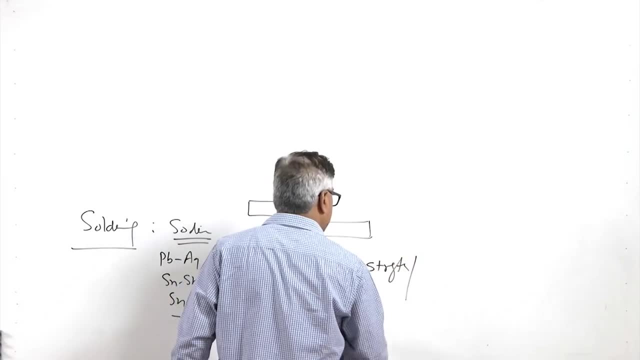 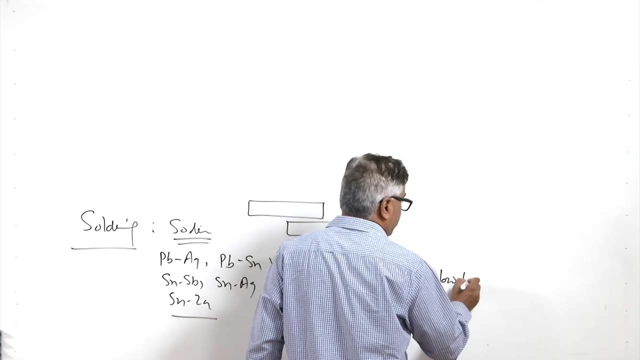 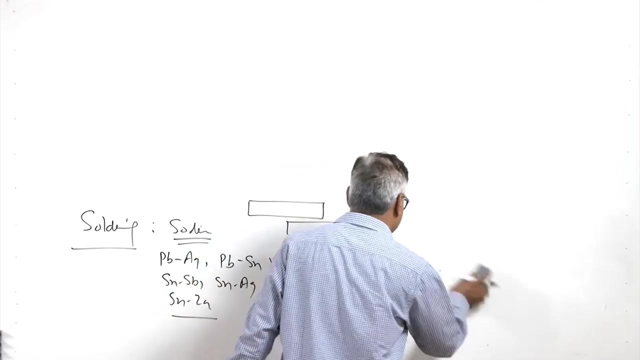 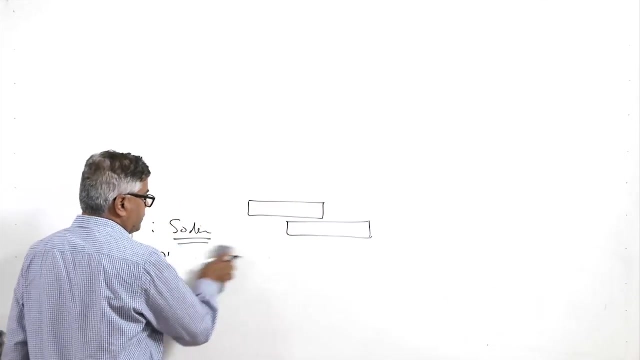 they are for the somewhat lower strength and the limited capability to withstand at high temperature. So they are good for the low temperature conditions. So these are low in strength and lower capability to withstand at a high temperature, Just like in brazing surface preparation. in terms of the shouldering, 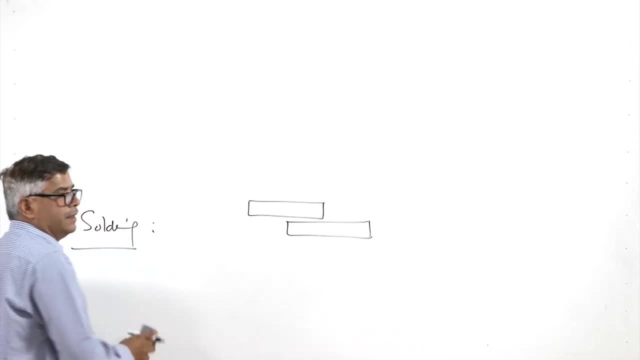 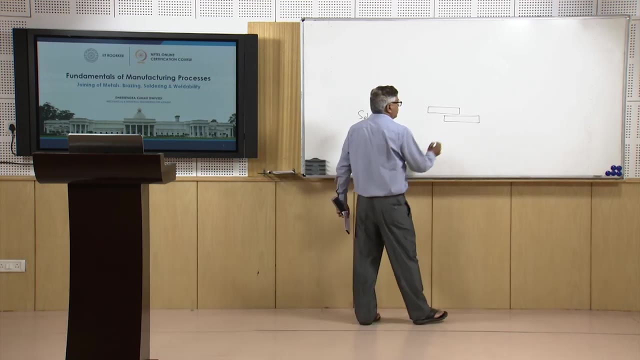 So the shouldering is done in terms of the cleanliness of the fink surfaces and the smoothness is important and the gap needs to be controlled very closely and for this purpose, the gap between the two is controlled in the range of, like say, 0.075 to 0.125 mm. and again this 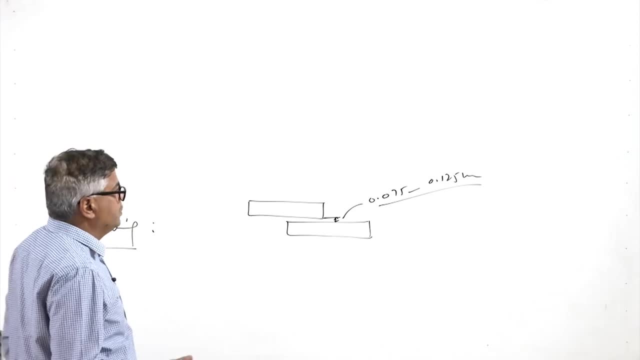 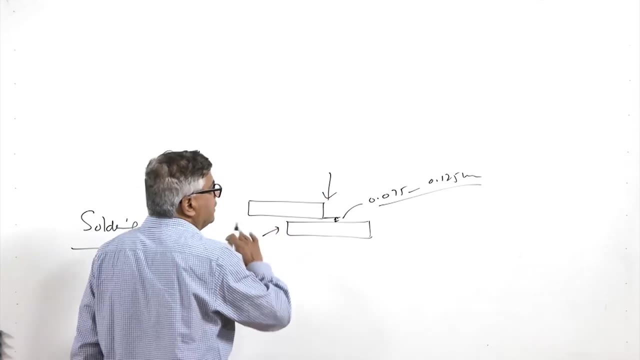 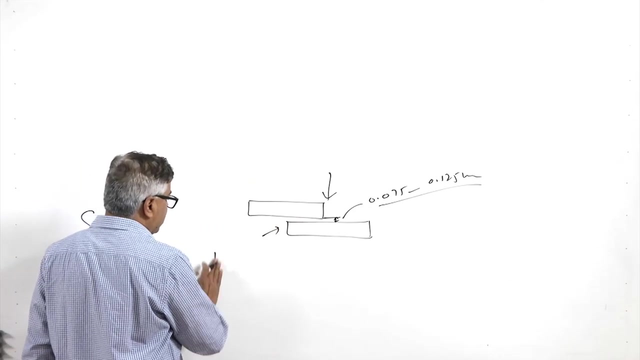 gap will depend upon the kind of shoulder which is to be used and is the surface conditions to be used. So obviously very low heat input is needed for melting the low temperature melting point shoulders. So this kind of heat camping, like shouldering iron can be used for. but likewise there are 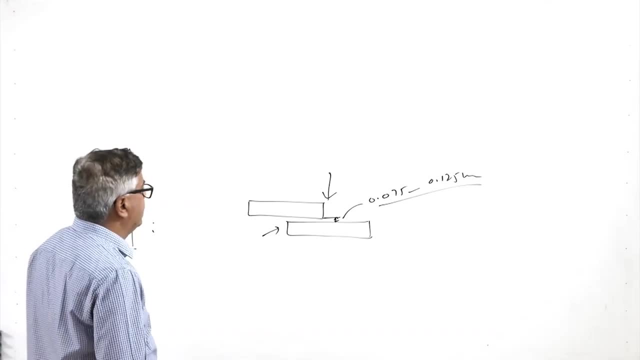 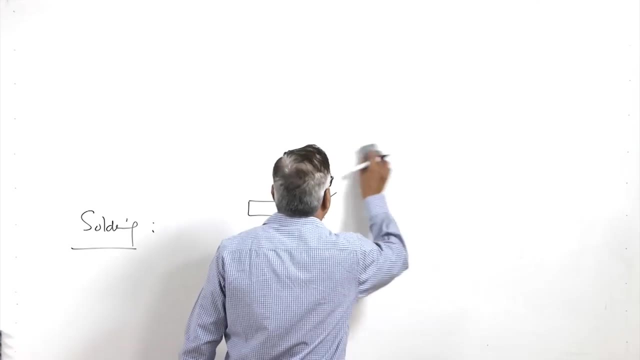 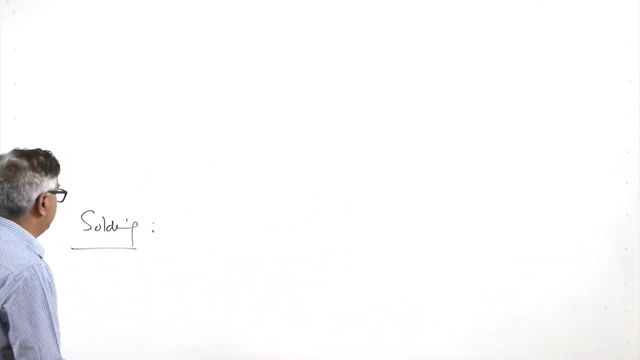 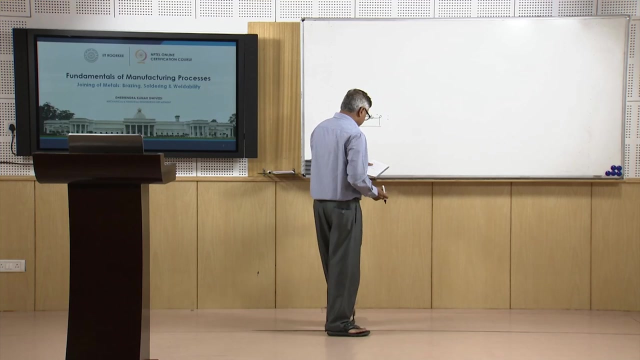 number of methods through which heat can be applied for facilitating the melting of the shoulder at the fink surfaces. so through the capillary action it gets distributed uniformly across the ordering 1.7 mm in the gap between the surfaces to be joined so that the joint can be made to improve the 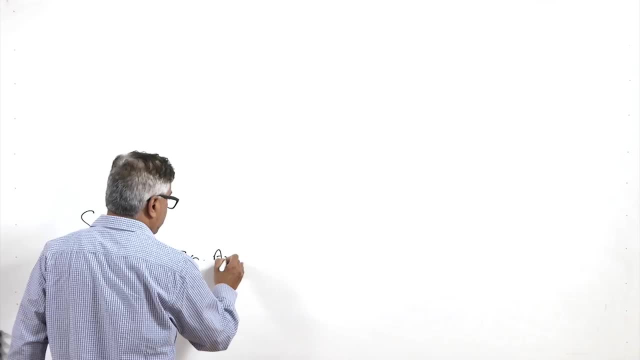 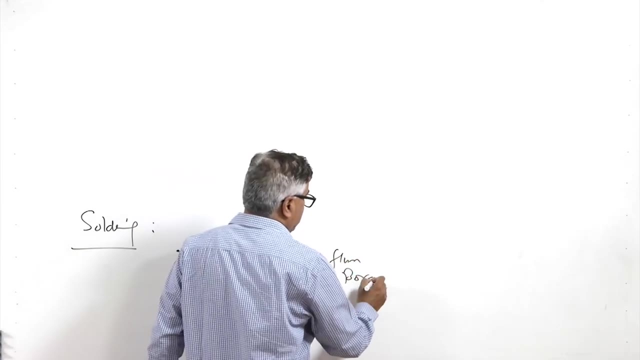 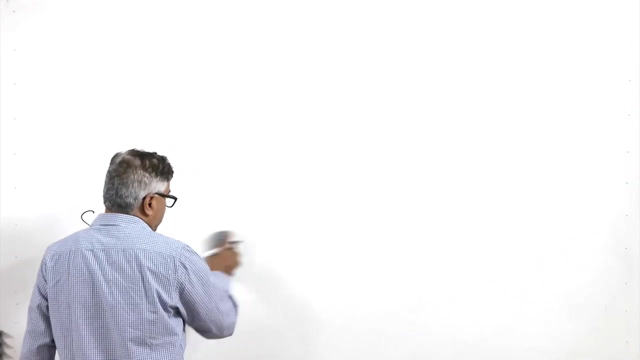 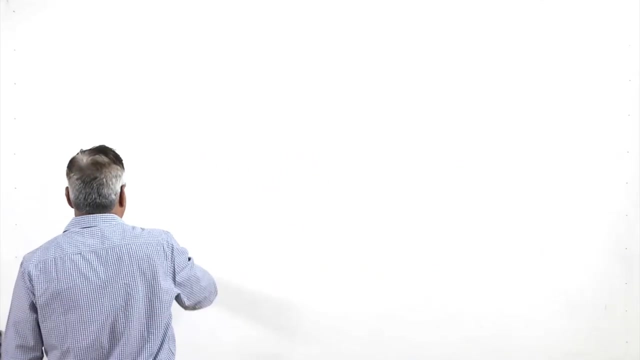 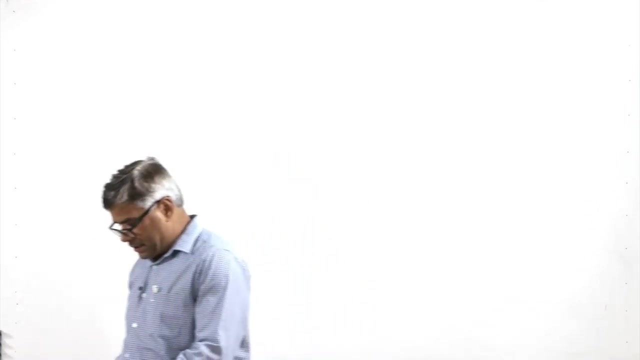 wettability, and normally the zinc and ammonium chloride is commonly used. Flux borax is another one which is used, but these needs to be cleaned properly so that then any kind of the corrosion effect on the joint performance can be avoided, because the residual fluxes can be harmful for the from the corrosion point of view of the base metal. 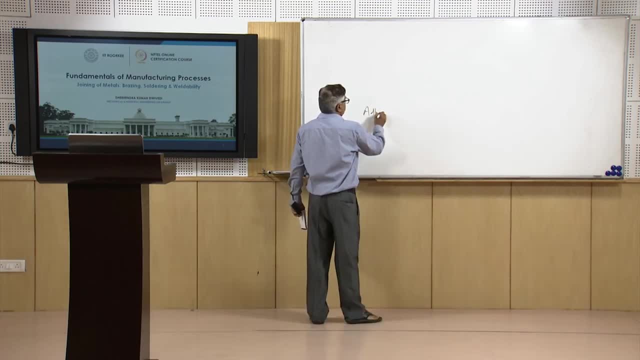 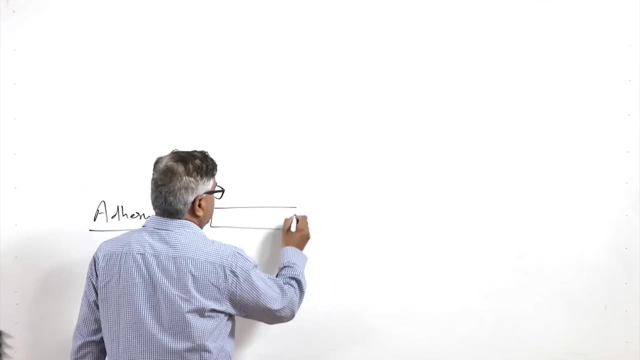 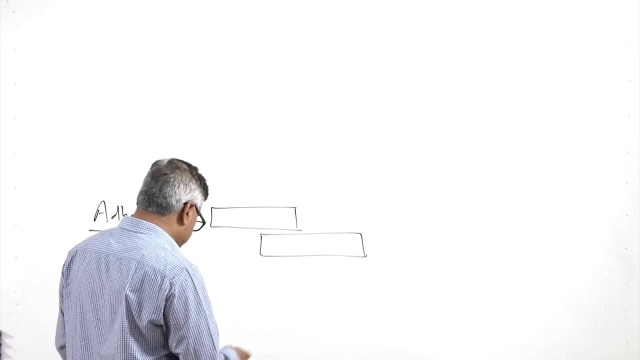 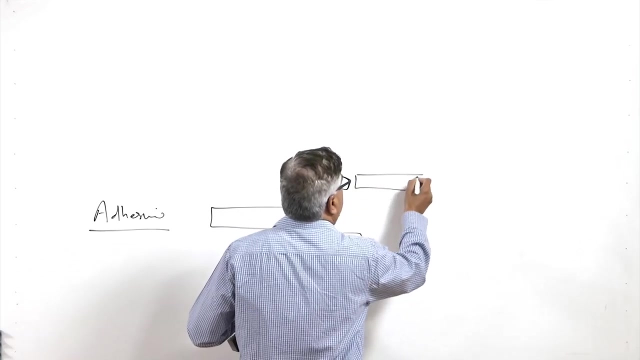 Now coming to the adhesive joints. adhesive joint is the kind of the involves the chemical bonding where in like the plates to be joined are kept in, normally in the lap joint configuration. but these can also be used in other joint configurations as well. Say, for example, the kind of joint configurations for this one, for the adhesive joints are also. 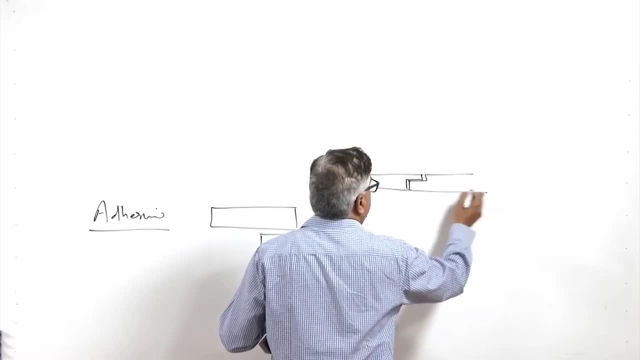 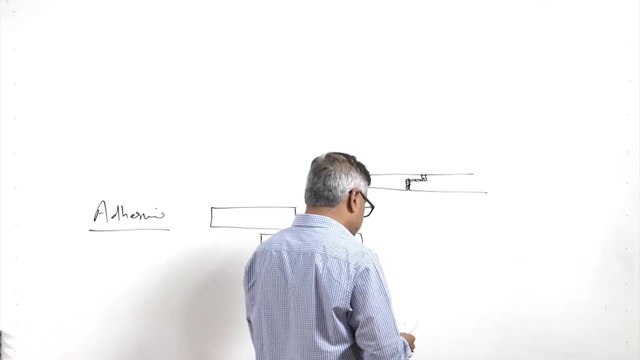 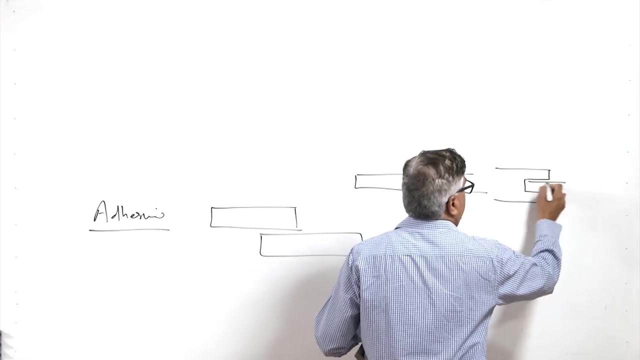 similar to that of the which were used for butt joint configurations, like adhesive spliced in this manner by making for increasing the joint surface area in butt joint configuration. Similarly that has another joint configuration is like this And here, So adhesive will be placed. this is the kind of components, so adhesive will be placed. 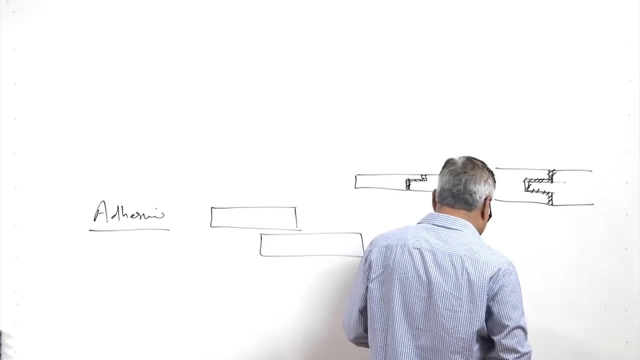 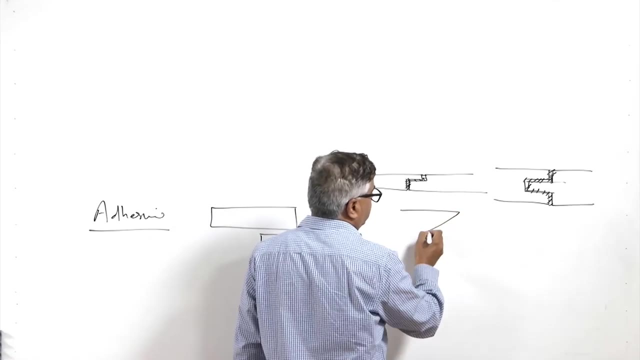 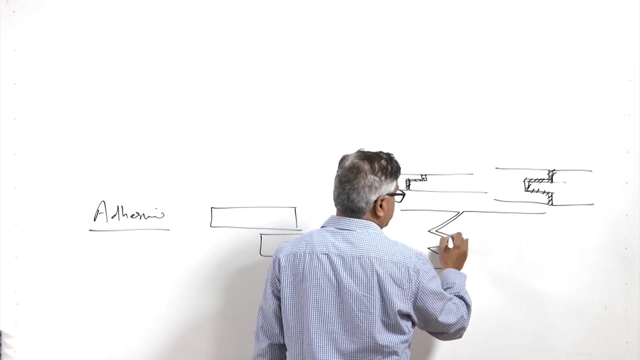 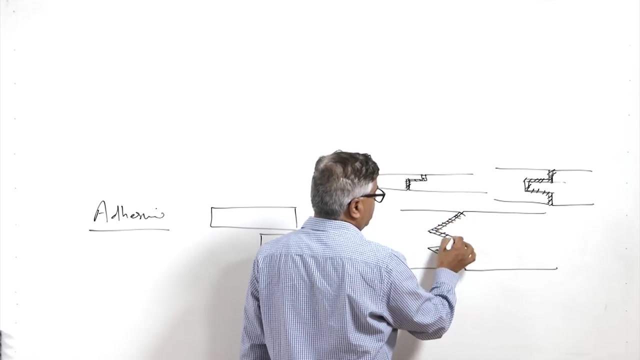 all around this surface area. So these are the methods which are used for increasing the area of the joint. like another one is like this: the component and another component having the configurations like this and entire this area is applied with the adhesives. so this increased joint area will be leading. 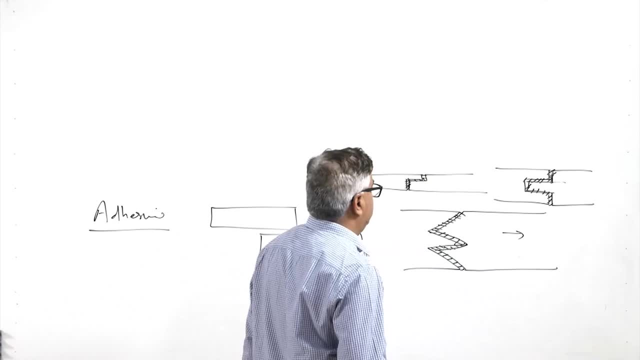 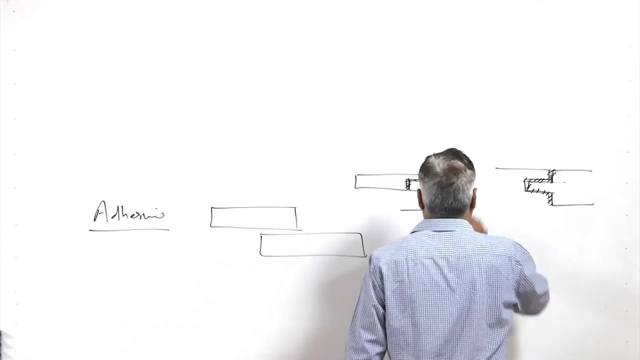 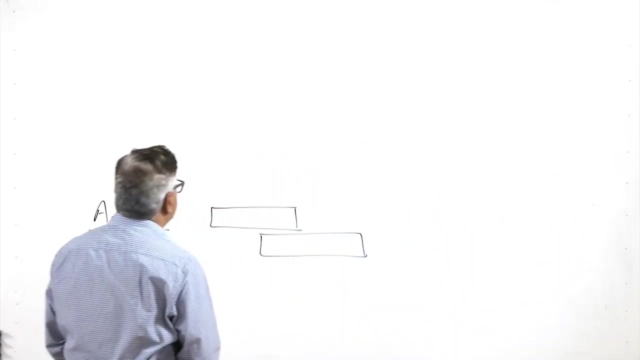 to the increased joint strength in the butt joint configuration. Likewise, the number of other kind of the joint configurations are there which can be used for increasing the joint surface area, but it is more commonly used for the lap joint configuration which is more simple, like this: 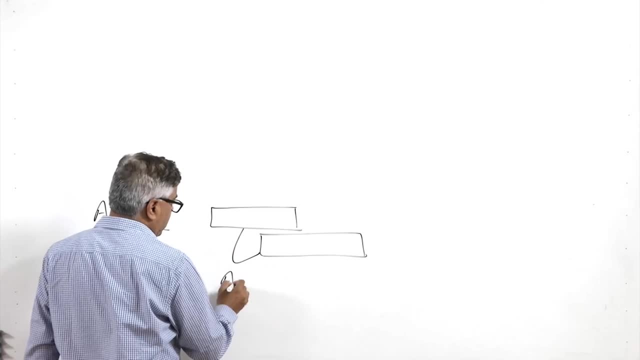 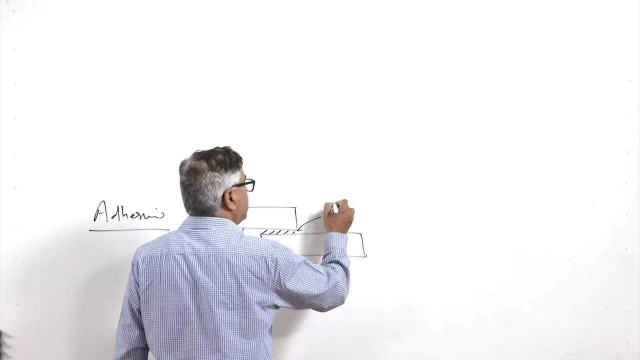 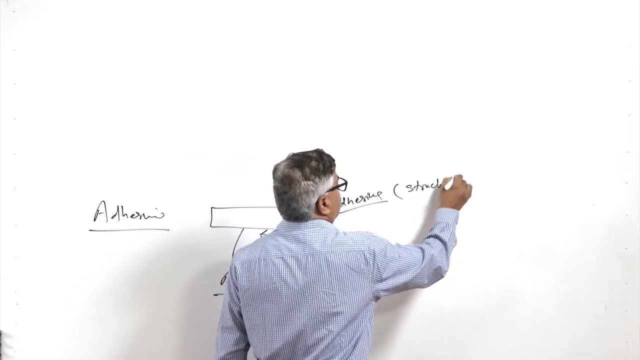 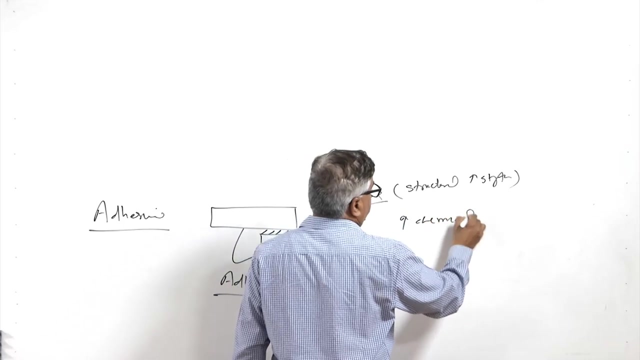 The components to be joined are called adherend and the adhesive which is applied between the finx surfaces is called adhesive, or the filler which is applied is called adhesive. Mostly this is structural adhesives for increasing the strength of the joint and basically the chemical reactions between the adhesive and the surface and the physical reactions between 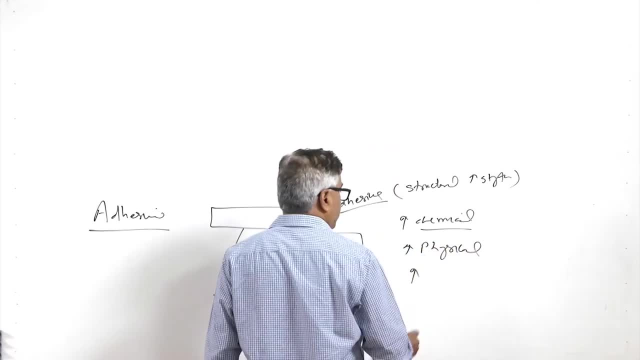 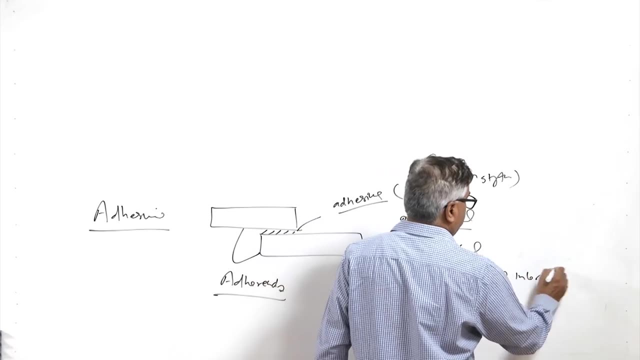 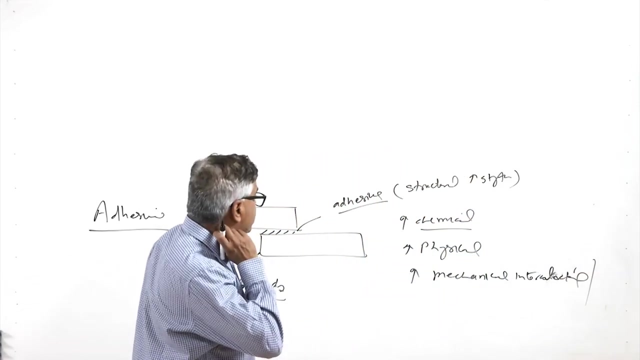 the adhesives. So these are the chemical reactions and the mechanical interlocking. mechanical interlocking: these are the three mechanisms. mechanical interlocking: these are three mechanisms which will be increasing the, which will be responsible for the joint strength. so some of these like 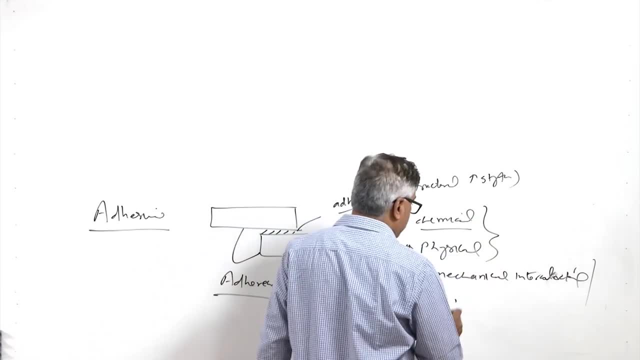 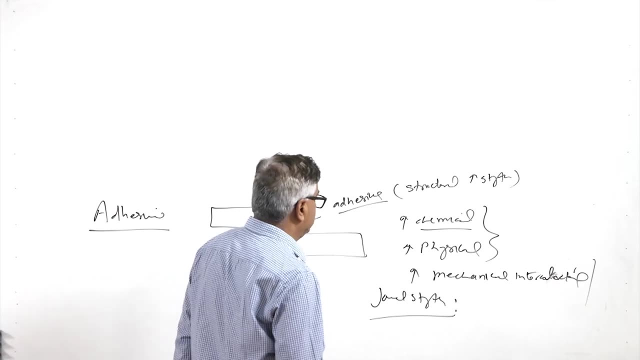 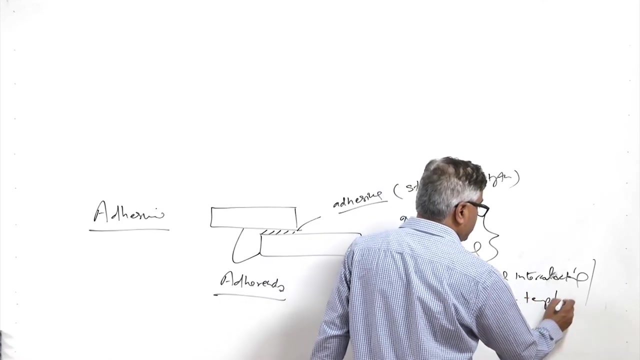 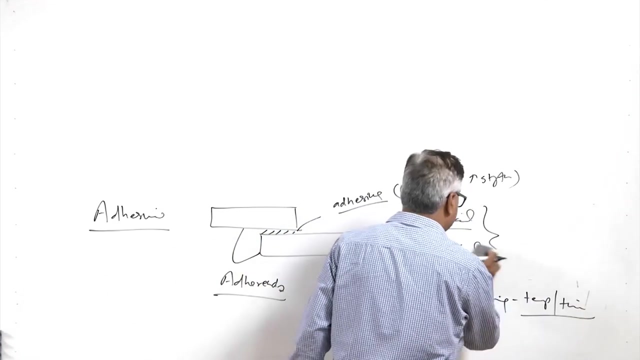 the chemical and the physical reactions which will be occurring after the solidification, after the hardening of the, after the hardening of the joint. and for this purpose, normally the curing is performed at a controlled temperature and the time. both these play an important role in ensuring the desired strength of the joint. So adhesive joints, joints are cured properly in order to have the reactions like adhesives during the curing. actually, curing increases the strength through the polymerization- this is one vulcanization- and condensation and condensation. so these things will be happening. 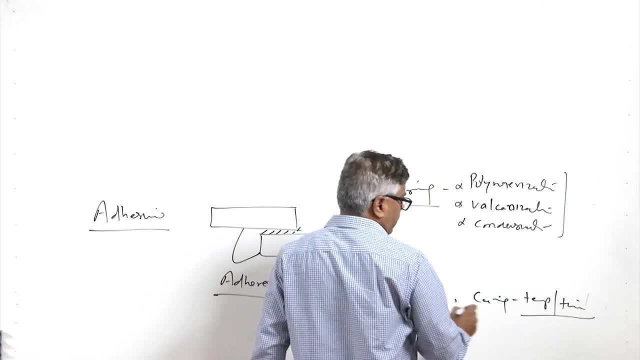 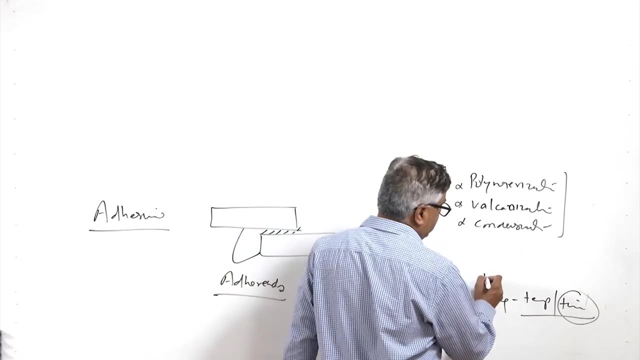 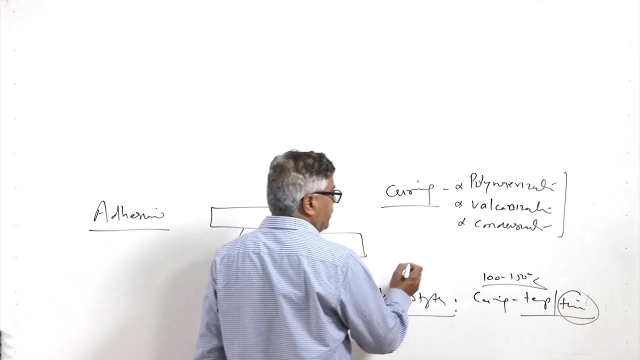 during the curing, And it is a, it is a, it is a. So it is important that curing is done under very controlled conditions of the temperature. normally like 100 to 150 degree centigrade temperature is used, and a curing should be done for optimum duration because otherwise it will lead to the under curing or over curing. In either case the strength of the joint will be less so. in case of under curing, when the curing has not been done up to for a proper time, then it will lead to the limited curing Reactions which will be occurring during the cure. curing and over curing can lead to. the thermal degradation of the adhesives due to the exposure at a longer period. So over curing can also be harmful for the joint strength, while as likewise, the under curing also adversely affects the joint strength due to the incomplete reactions and the reactions which will be occurring during the curing, like vulcanization, polymerization and condensation. 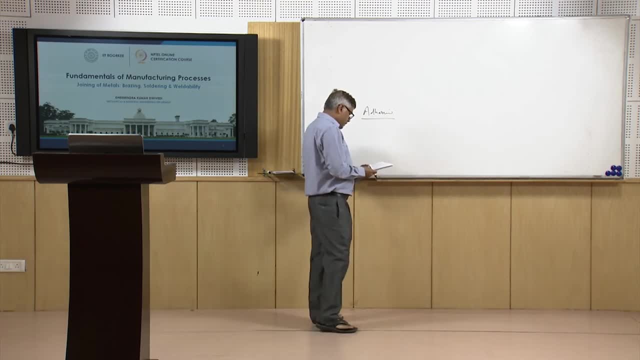 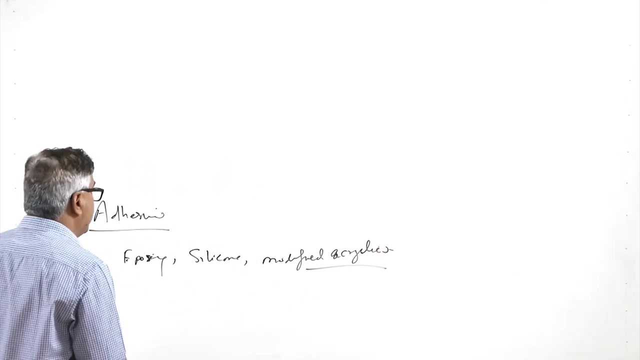 So the common kind of the resins which are used for developing the adhesive joints are like epoxies, epoxies and silicon, and then modified acrylics, Modified acrylics, Modified acrylics. So these are the things, as we have said, for uniform spreading of the adhesives, it is important.